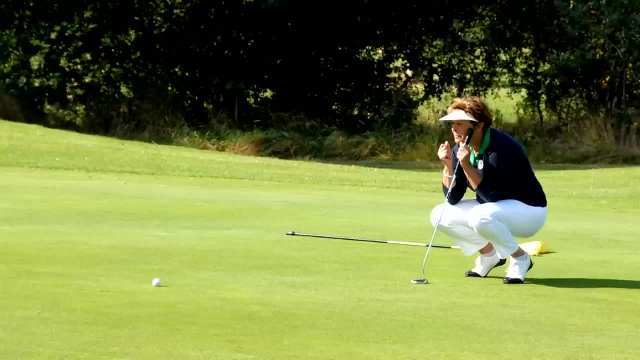 We're pulling for you, Sally. Don't know if you actually got the ball in the hole, but we're pulling for you, Sally, You can do it, Sally, You can do it. You see, she's so excited She doesn't know. 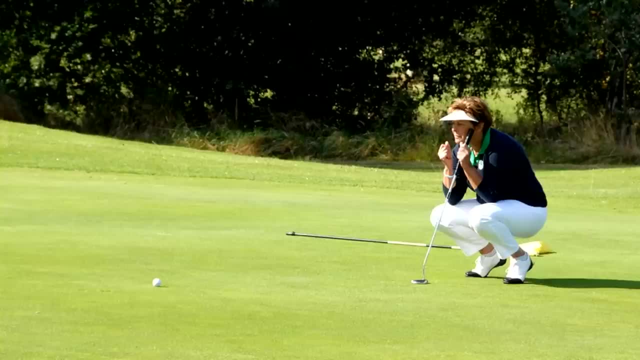 She doesn't know, but we don't know either. So anyway, All we can do is guess. We don't really know. We don't know Sally all that well, but let's pretend that Sally loves golf, and let's pretend. 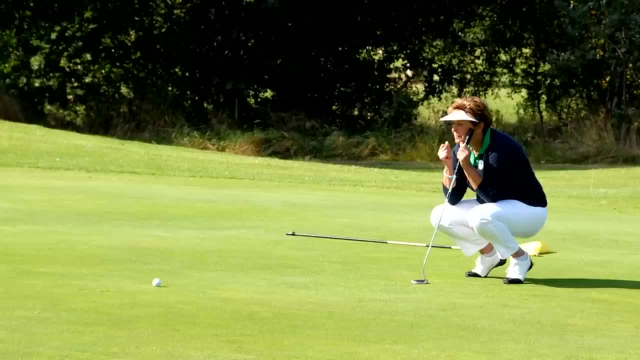 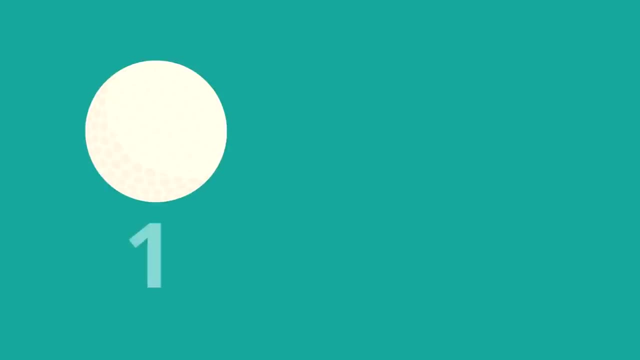 that Sally likes to collect golf balls. So Sally is playing with one golf ball. Let's say that's the only golf ball she has with her right now. She's got one golf ball, but she finds another golf ball by a tree. 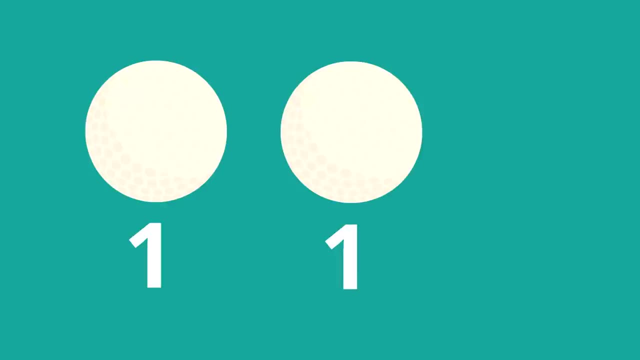 So she had one golf ball and then she found another one. We need to put these numbers together, don't we, to find out how many golf balls she has now Putting numbers together, That's addition, That's addition. So now we put these two numbers together. 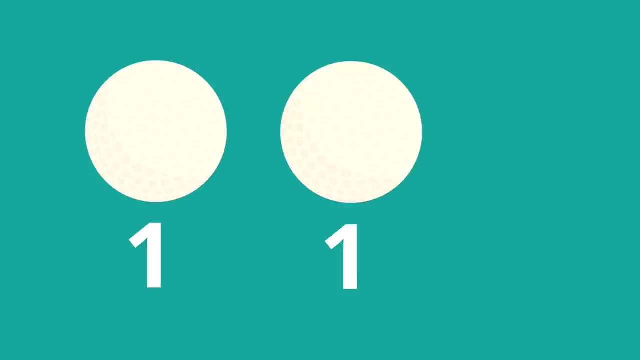 She had one golf ball. She found another one, So let's add both of those numbers together. She found another one, So you're adding both of those balls. How many do we have? Yeah, two, Sally now has 2 golf balls. 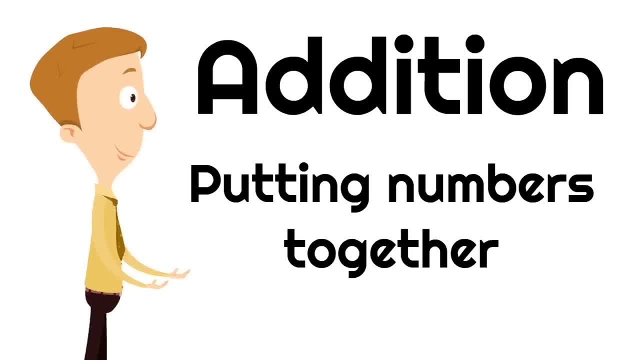 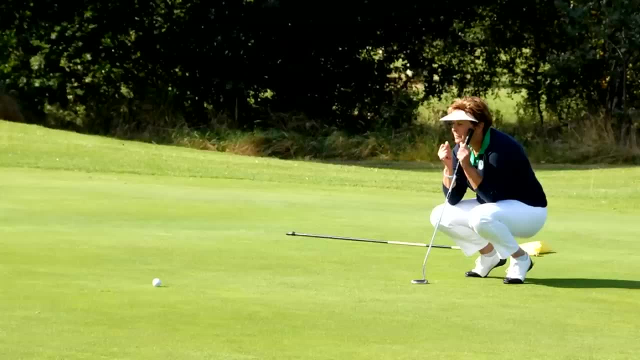 Good job, Sally. Oh addition, I knew I loved you. Oh addition, All you are is just putting numbers together. So simple, So fun A game anyone can play. Well, you know where we're going, old guys. 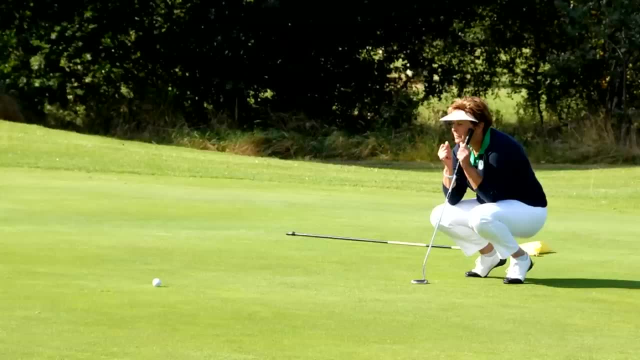 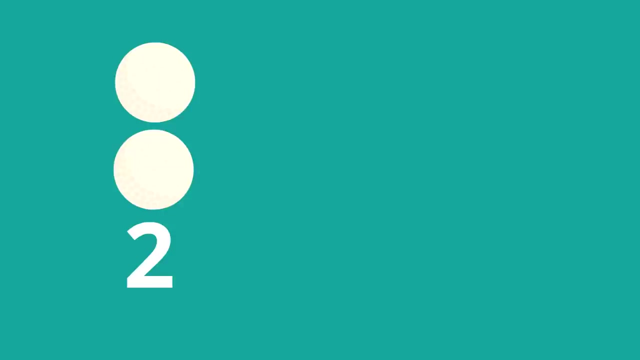 Tour Song: производs music. We're about to give you開始. You can�, Sally. you know, Sally. she went back to that golf course the very next day because remember, she loves golf, right, and of course Sally brought her two golf balls because remember she had one golf ball, then she found another one. so 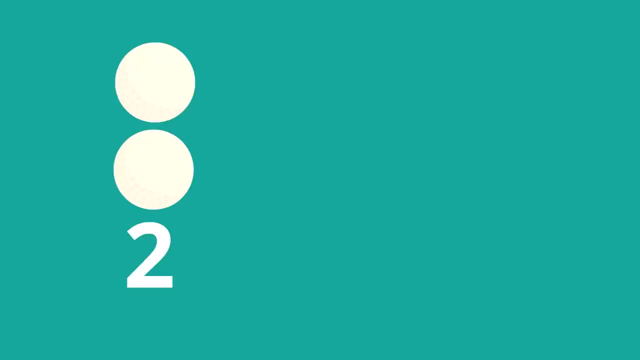 now she has two. but you know what? she had a great day at the course and she actually found two more balls. no, crazy, sadly, is really great at finding golf balls. she found two more balls. now we have to find out how many golf balls she has. wait a second. oh, we're putting that. we're putting numbers together, it's. 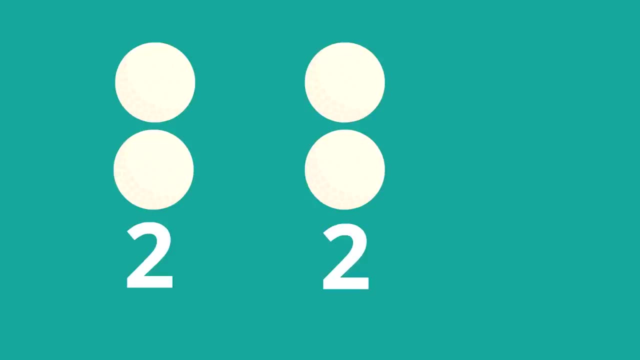 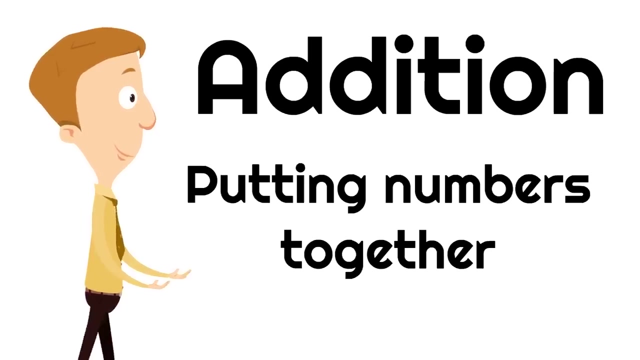 addition. it's time we're gonna get to do addition again. remember, addition is putting numbers together. she had two more balls and she found two more balls. and now she's found two more balls and we get to find out how many she has. now that's addition, putting numbers together. so she had two balls and she's found two. 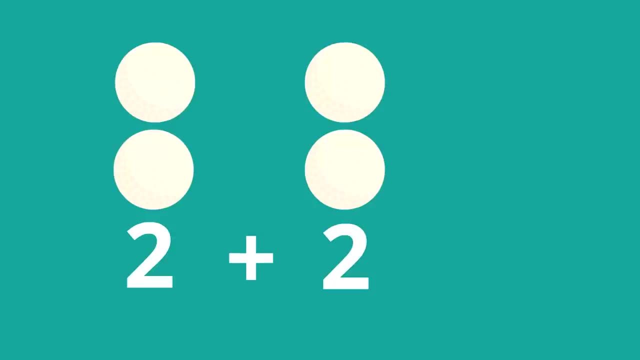 new ones. so we need to find out what two plus two is. what a great addition problem. what's two plus two? if you don't know, you can actually just count the golf balls. what's two plus two? two plus two, yeah four. two plus two equals four. remember, addition is putting. 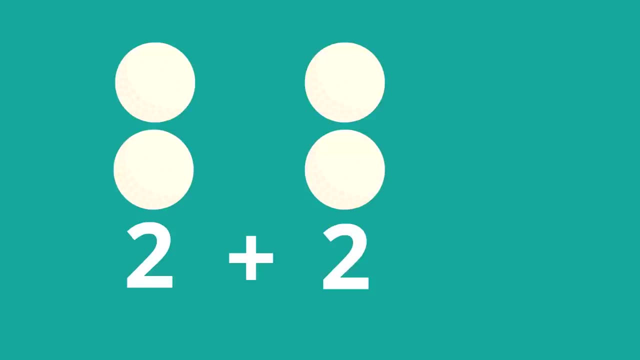 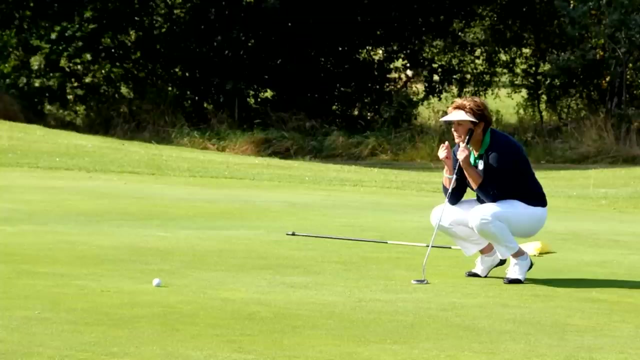 numbers together: two plus two equals four. that's addition, putting numbers together. oh, bless her heart. Sally's at it again. she's back at it to главное. she's: Ya whoops, I got it right. she's back at it. she's going back toTransform. she's saying: it's like: why are you doing this the next time you go? 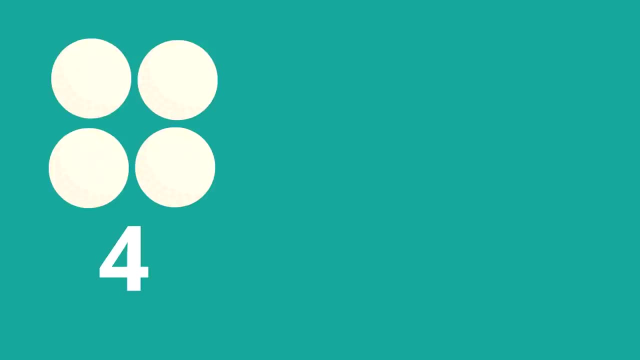 back here in a day or two is one of those Catch the Balls mind yelling Villains. shut up. okay, she's dead, she's back at it. yeah, now let's see how she got four hands. no one did. she was the one that got the most balls. yeah, she's definitely. 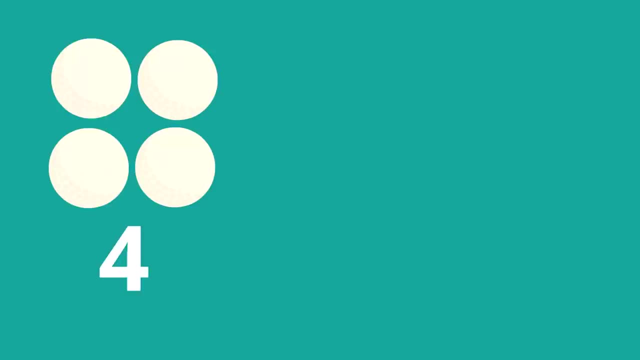 got the most balls on the Monica. if she did, she's in into theск huge. Now we need to figure out how many golf balls she has and, yes, we're putting numbers together, So it's going to be an addition problem. She had four golf balls and now she has three more golf balls. 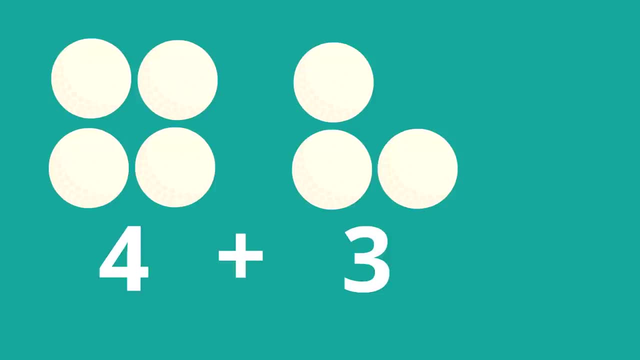 So what is four plus three? Remember, with addition we're just putting numbers together, So if you need help, you can actually count the number of golf balls on the screen. What's four plus three? Yeah, four plus three equals seven. She has seven golf balls now. Great job adding. 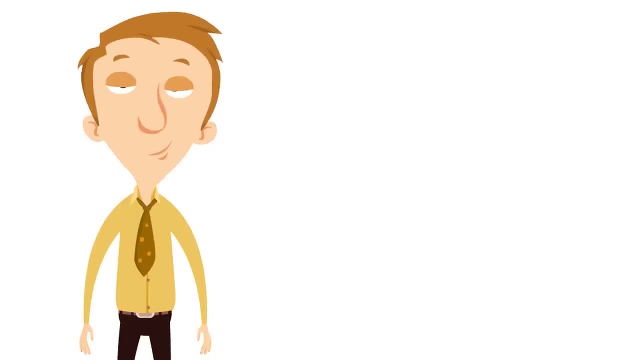 Well, now you know the basics of addition and now you know what I love addition so much. in the comments below, Tell us how much you love addition. because it's fun. right, It's simple, It's fun. Where's Sally? Where's Sally? 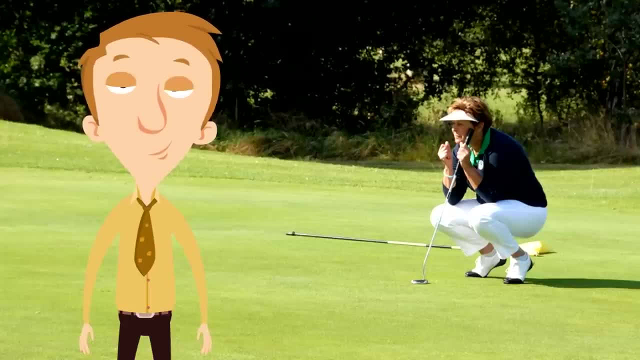 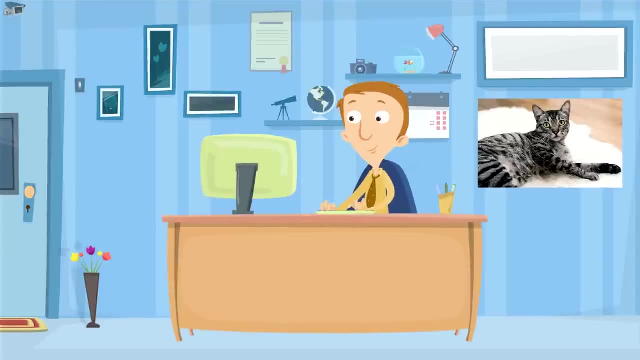 Thanks for helping us count how many golf balls she got and remember. addition is just putting numbers together. We are so happy to have you with us. I mean, you are so awesome, You really are. Oh, you like my poster. Yeah, mr Whiskers poster, you know, it's pretty cool, Pretty cool, you know. 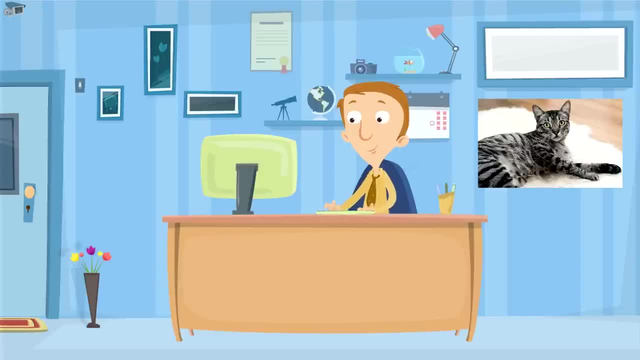 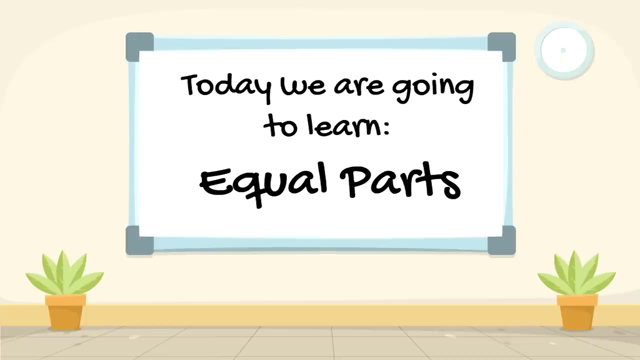 It's a pretty cool poster, pretty cool cat too. I wonder what he would like to learn about next if he would learn from one of our videos. What would he like to learn next? Hmm, How about? Hmm, let's learn about Equal parts. we're gonna learn how to recognize. 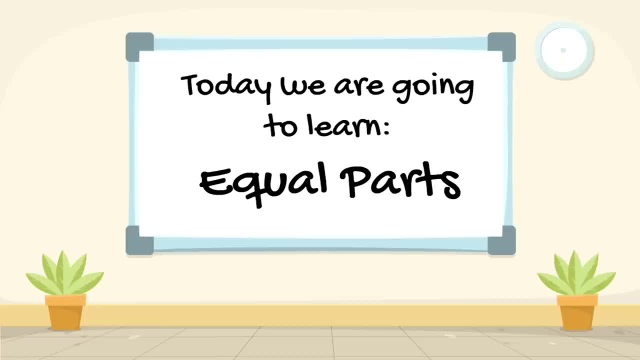 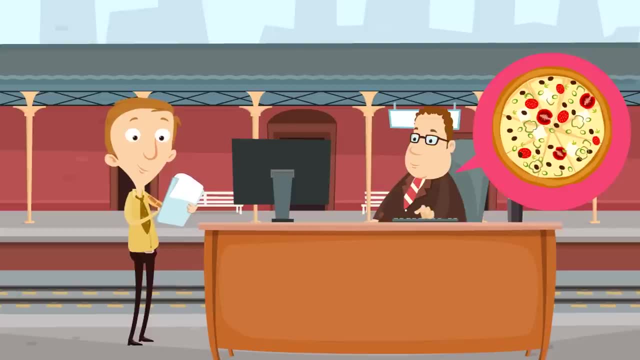 if something shows equal parts or if something shows unequal parts. Hold on, my My boss is giving me his pizza order again. I'm telling you he loves pizza Way too much. I mean, I like pizza, It's fine, But he's always giving me his pizza order. I'm always picking it up for him and 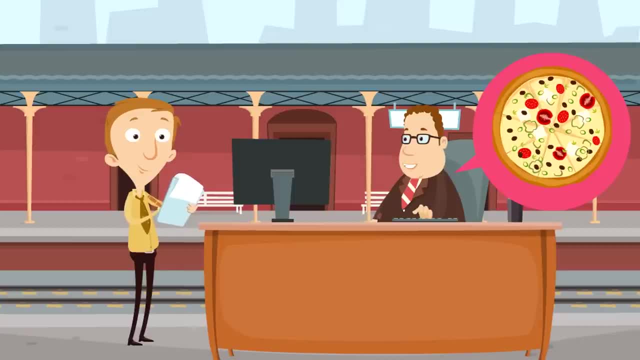 This is just this is you know? I just Here, I just gotta keep writing down. you know he's got all these instructions. He likes his pizza a certain way. Oh Wow, Oh He's, he wants, he wants me to have some of the pizza with him, Oh. 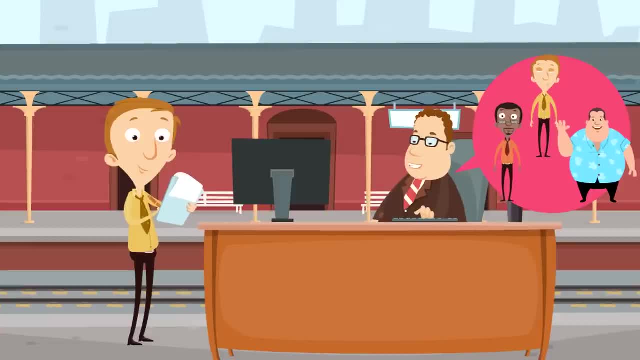 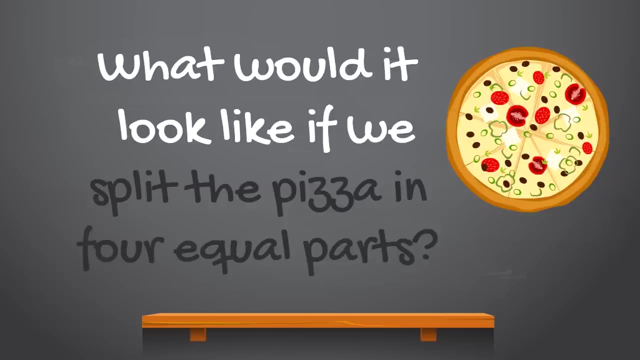 Man and and Ted and Gilbert- Oh, all four of us having the same pizza, all the sharing a pizza. So what would that look like? what would it look like if we had This pizza put in four equal parts? How would we know that these parts of the pizza were equal? a? 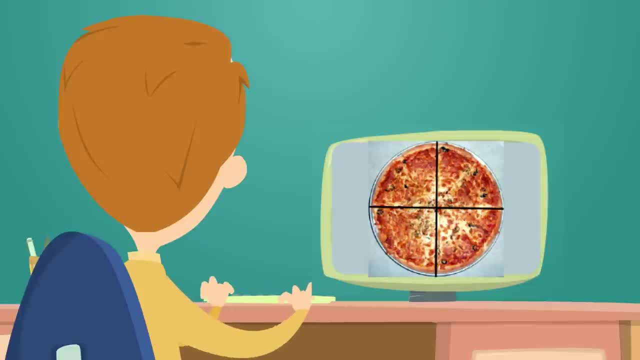 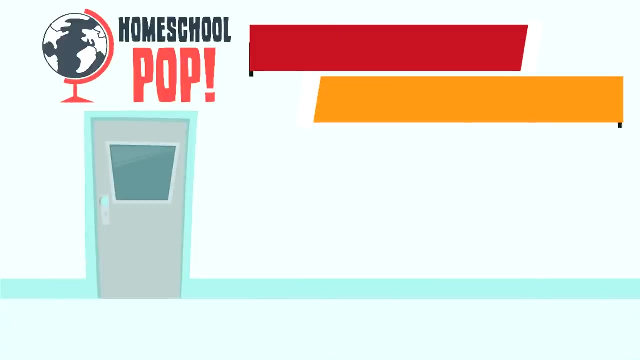 Pizza with four equal parts might look like this. Pretty cool, huh? We know the parts are equal because each of the parts are the same size. a A pizza with four equal parts might look like this: I'm going to play a game called: are these equal parts? 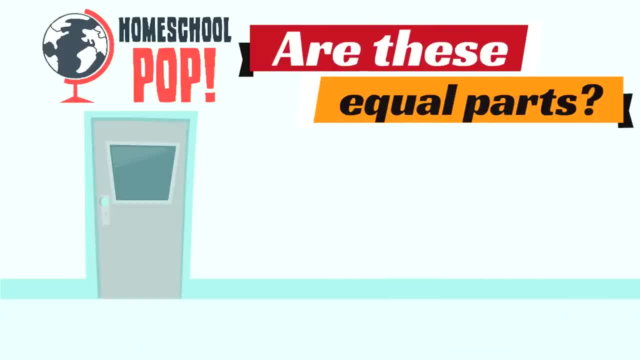 Okay, it's not really a game, but we can make it into a game, right? Okay, it's not like checkers, It's not like chess, you know. it's not like basketball, like soccer. Okay, It's not like a game, game, game. 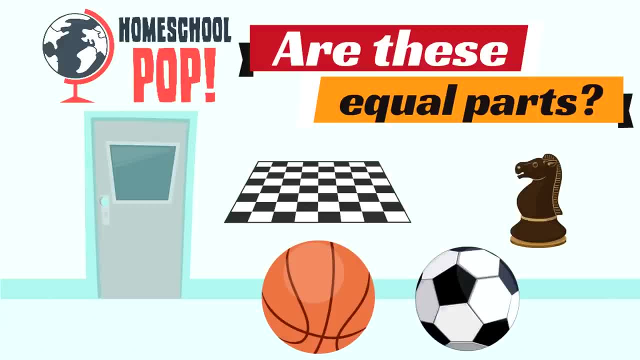 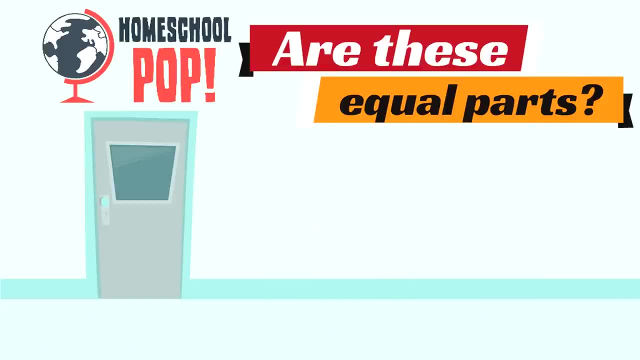 Okay, but it's still gonna be fun and we're gonna be able to see work with me here. Okay, we're gonna be able to see if, if these pictures show equal parts or if these pictures show unequal parts. so here is our first picture. now we're gonna be looking to see if this picture 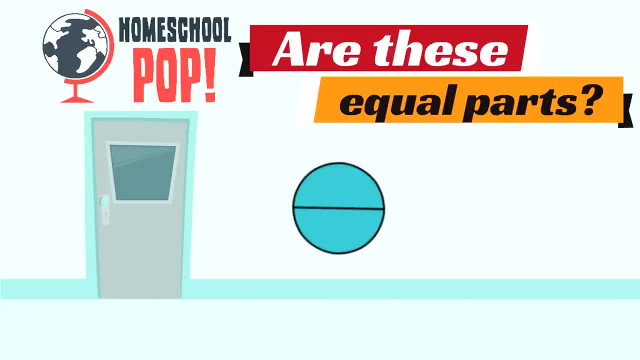 shows equal parts, and this picture shows how many parts. two good job. now are these equal parts? yes, this picture shows two equal parts, and we know they're equal because they're the same size. now look at this one. this picture shows how many parts. yeah, three parts. now are these equal parts? 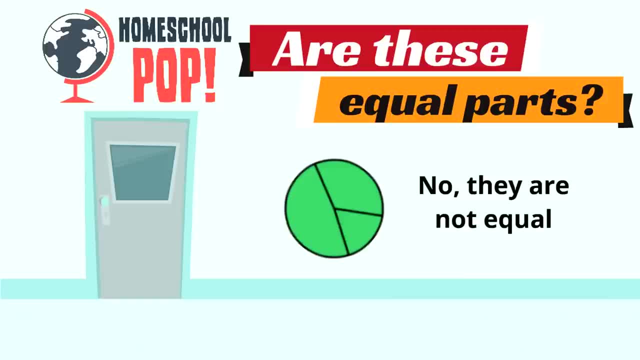 no, they're not equal parts. they're not equal parts because they're not all the same size. this picture does not show equal parts. great job. now let's give this picture a try. how many parts to this picture show three? good job, and are these parts equal parts? 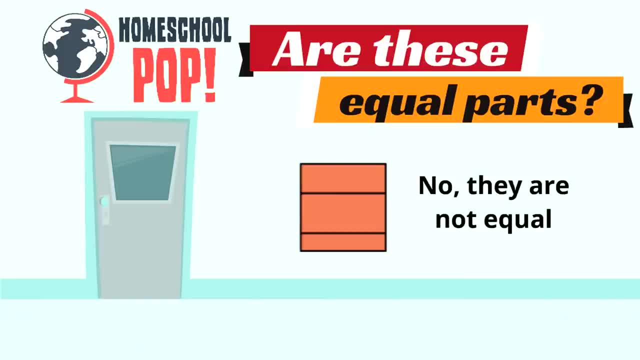 no, they're not equal parts. can you imagine if you've got that bottom part, if this, if this square was like a cake and you got that bottom part? that wouldn't be fair why these are not equal parts. let's give this triangle picture a try. how many parts does this picture show? great job, three. and are these equal? 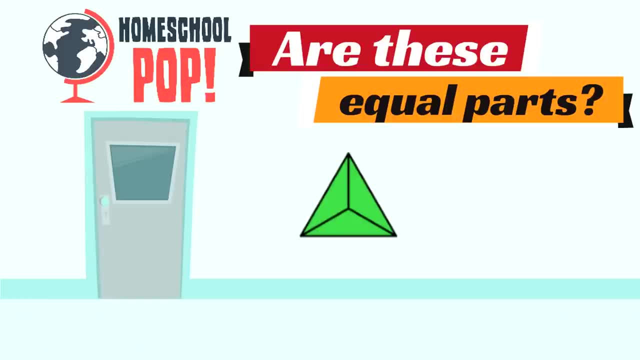 parts? Yes, they're equal parts because they are all the same size. Equal parts means each part is the same size. Great job. What about this picture? How many parts does this picture have? Be careful when you count. it's a little bit tricky. 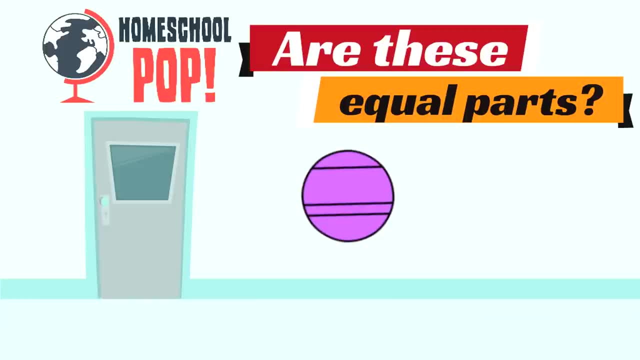 This picture has four parts. Now, are these equal parts? No, they're not equal parts. How do we know? Because they're not the same size. I don't know about you, but I feel pretty good about this equal parts stuff. 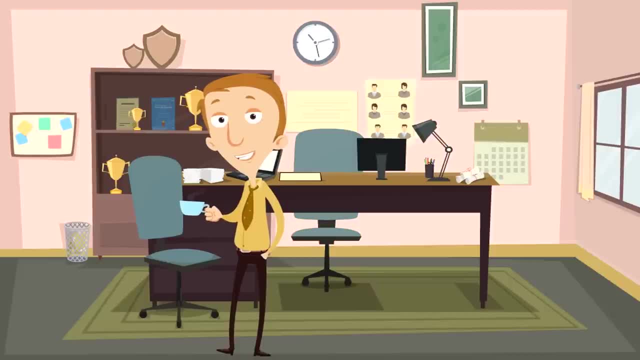 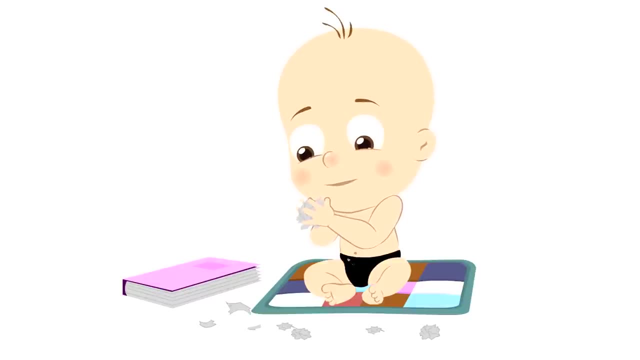 It just means that the parts are the same size. When they're the same size, that means they're equal. Oh, this little baby's putting together a little thing, A little craft. Oh, it's so great. I just love that. that's so good. 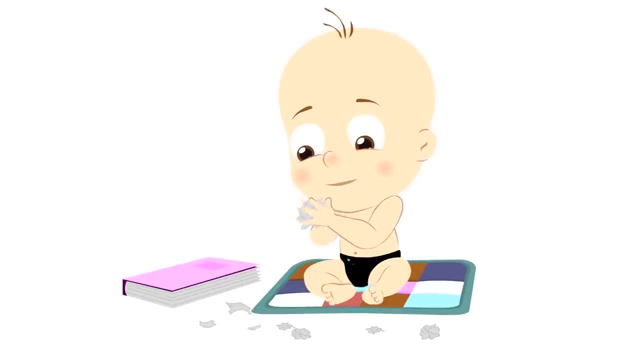 Wait a second. that paper's from that book, isn't it? Okay, see, this is not an approved arts and crafts activity right now. Okay, we're going to have to take care of this, but first let's learn about subtraction. 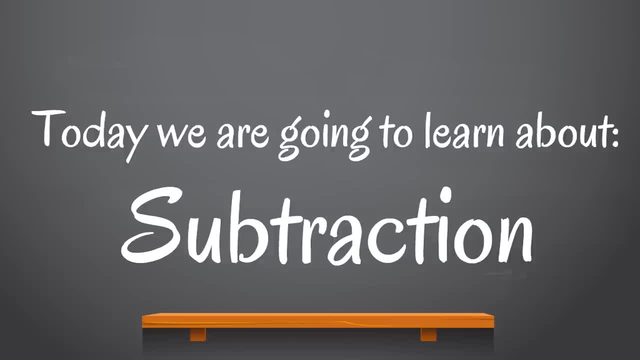 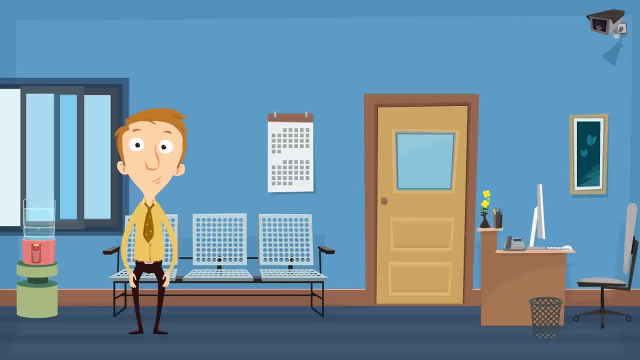 Do you know where I am? Yes, you know. I'm waiting patiently in this waiting room. Oh man, it has been a while. Have you ever been in a waiting room before? Cool, Yes, they can be fun, but you do have to be patient, and it's a good time to think. 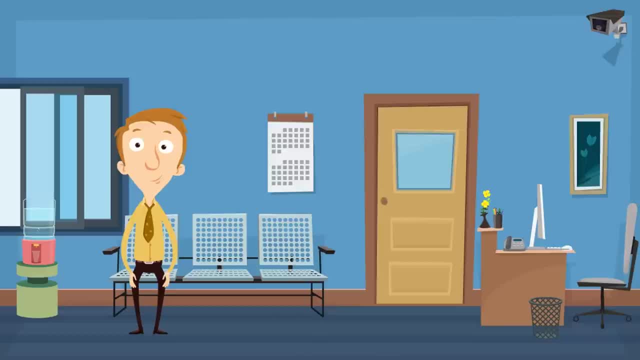 You know, you can think about all kinds of things, Like, okay, I have 8 fingers. Okay, Okay, cowboy hats. i know it's crazy, it's weird: eight cowboy hats and they're all the exact same, the exact same hat. i've got eight of them, eight brown cowboy hats. i mean, what's a guy gonna do? 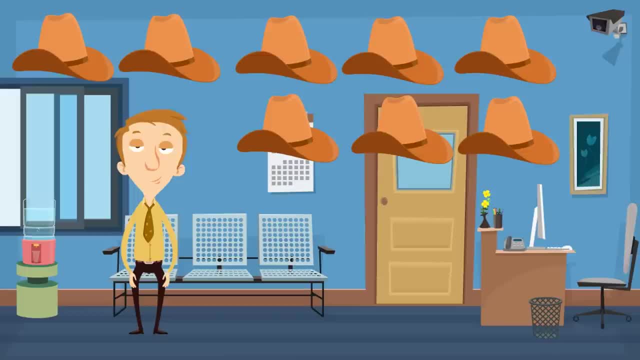 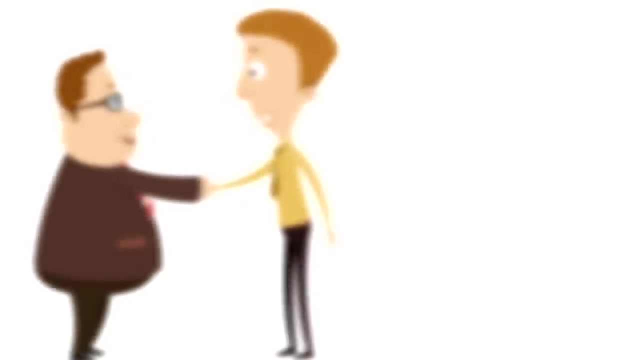 with eight brown cowboy hats that look the exact same. what could i possibly do with eight brown cowboy hats that are all the same? i mean, i should probably give some of them away. you know, i could give away one of my hats to bob, and cookie might want one. yeah, she might like a brown cowboy hat. 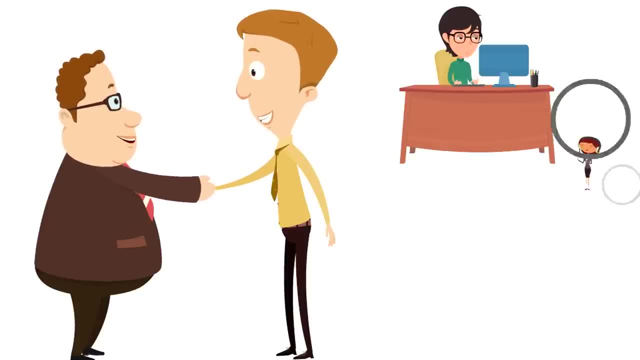 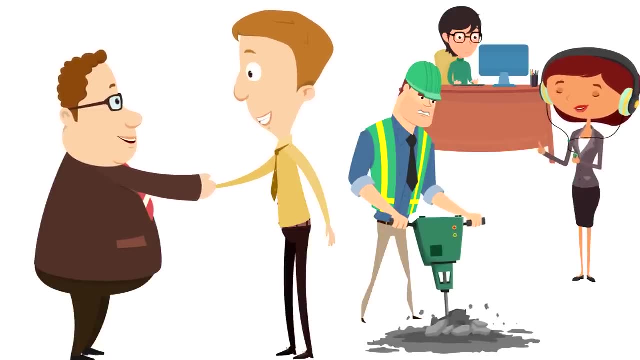 you know i could give one to nancy, you know, just in case she ever got invited to a western party and chomsky he'd take a hat. so as i'm sitting here thinking about my eight hats, i need to figure out how many of them are the exact same hat. i've got eight brown cowboy hats that look the exact same. 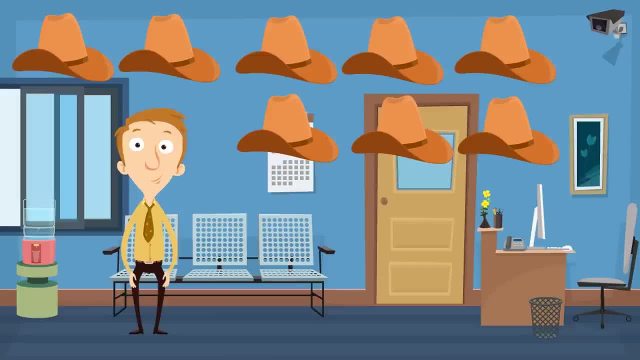 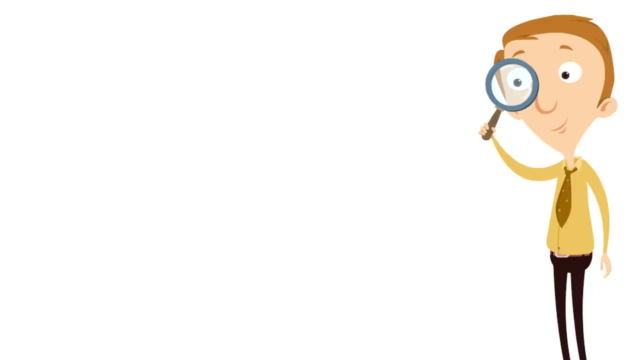 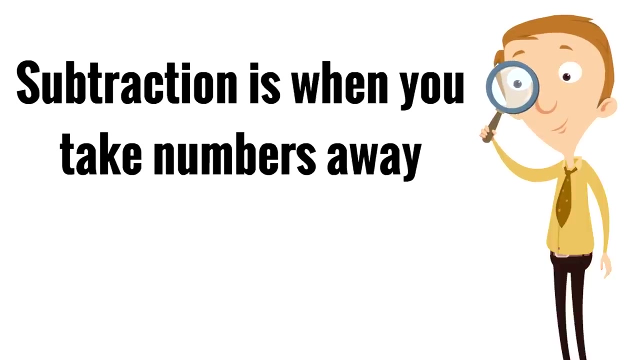 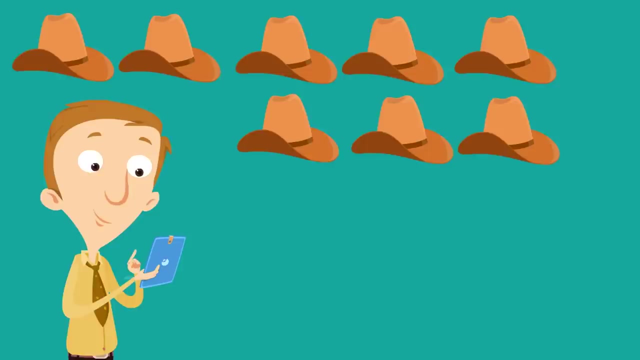 how many hats i'll have left if i give some of them away. to figure that out, we need to use subtraction. you see, subtraction is when you take numbers away. yeah, very simple, subtraction is when you take numbers away. so i begin with eight hats and i decide to give one away. we're going to need 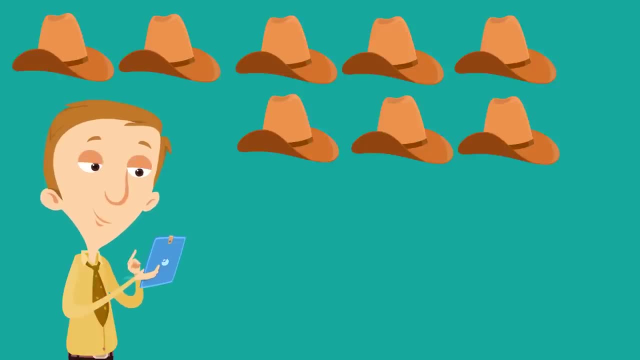 to subtract one from eight. the way we would write this is eight minus one. now remember, when we subtract we're just taking numbers away. so eight minus one, we're going to just take one away. there we go. how many hats do i have left? what is eight minus one? if it helps you, 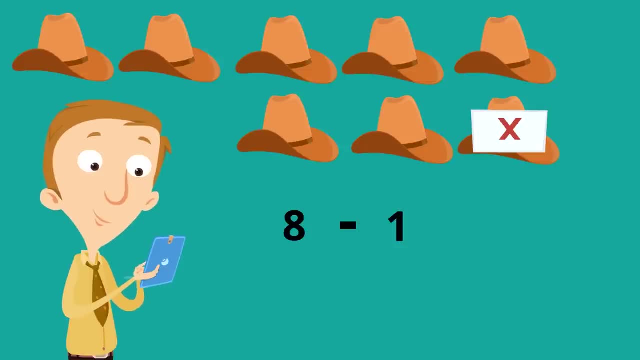 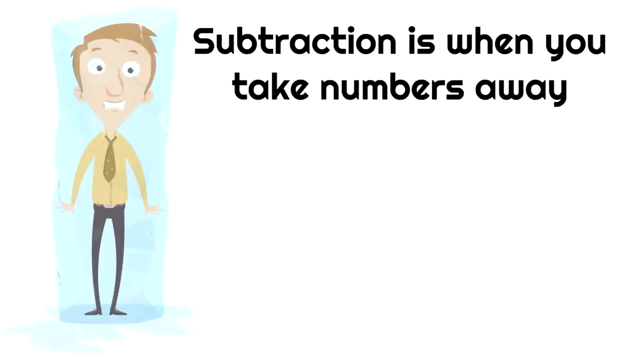 can just count how many hats i have left. what is eight minus one? yeah, seven. eight minus one is seven. now i have seven hats. remember, subtraction is when you take numbers away and, as you might have noticed, we use the minus sign when we write a subtraction problem. you can see it right there in the middle. it's just like a dash. that's the. 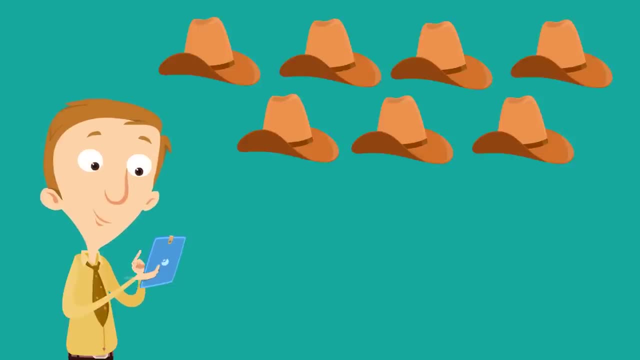 minus sign. So now I have seven hats, but two of my friends stop by and I decide: you know what? I know? I just have seven hats now, but I want to give two of them away. Now I'm going to be subtracting two hats from my collection. 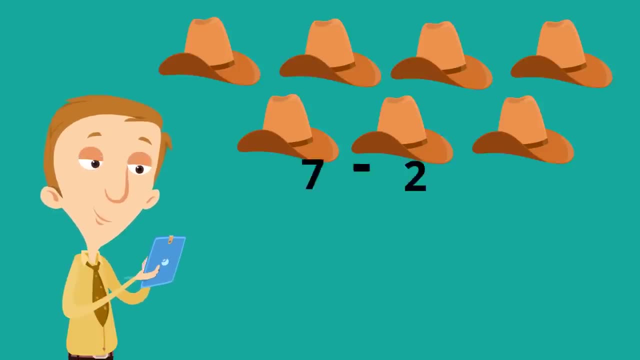 We would write this by saying seven minus two. Now, let's take away two hats, We'll find out how many we have left. What a wonderful subtraction problem. What is seven minus two? If you need help, you can just count how many hats are left. 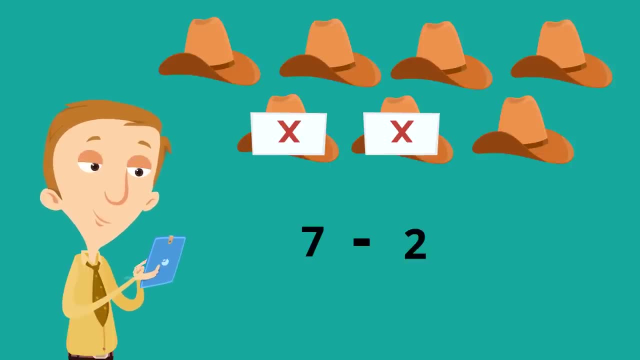 What is seven minus two? Seven minus two equals five. yeah, five hats, and you can even count them: one, two, three, four, five. there are five hats left. Seven minus two equals five. Do you see how fun and simple subtraction is? 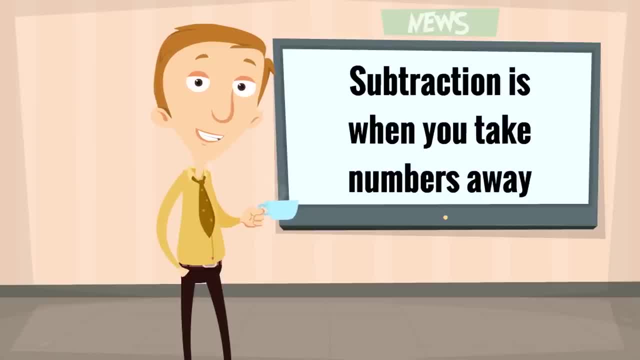 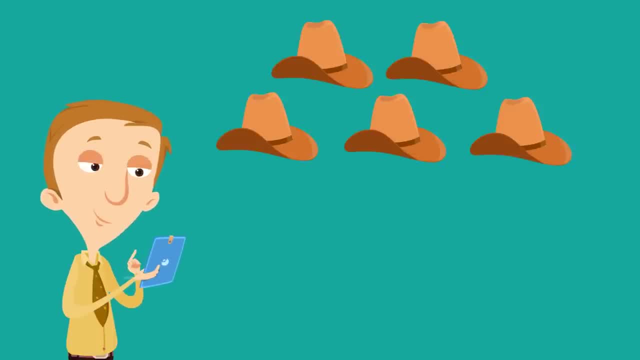 Subtraction is when you take numbers away. So now I have five hats in my collection- only five hats left. But then I meet up with my cousins Hooey, Dewey and Stewie, who want to have hats too, and I'd love to give them hats. 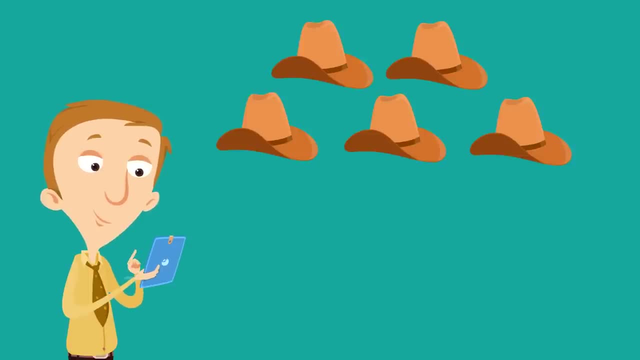 So I'm going to give three more hats away. So I have five hats and we're going to subtract three hats. We would write that five minus three. So now I have five hats in my collection. Only five hats left. Oh, I love subtraction so much. 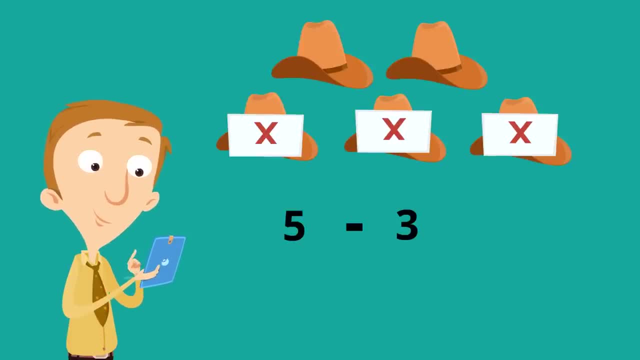 All right, bada bing, there we go. The three hats are gone. So five minus three, how many hats are left? It's pretty simple, isn't it? Yeah, five minus three equals two. Good job, Subtraction is just taking numbers away. 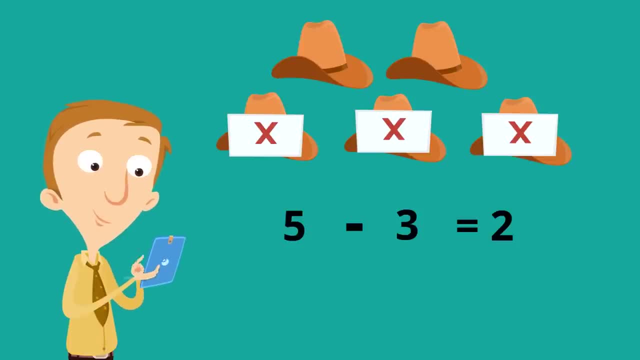 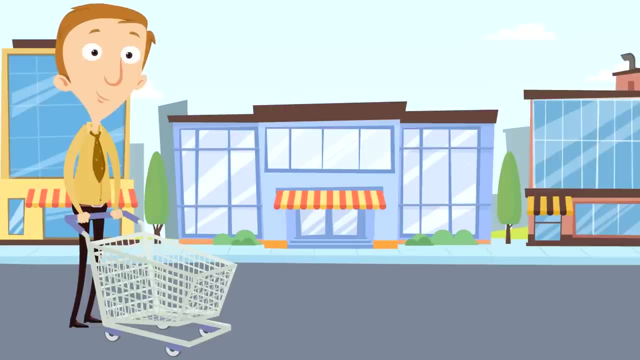 And five minus three leaves you with two. Now I have just two hats. We love subtraction. I mean subtraction is when you take numbers away. And why am I in the middle of the road with a shopping cart? So I have my two hats. 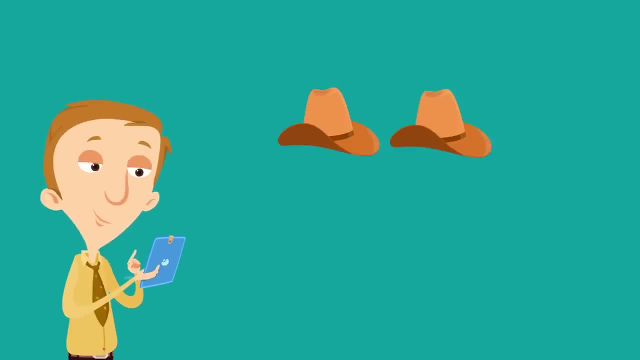 And that's fun. Subtraction is when you take numbers away. Subtraction is when you take numbers away, You don't have to keep the number on your bus And you don't have to implement it two times. You don't have to go through the top of a bus ever. 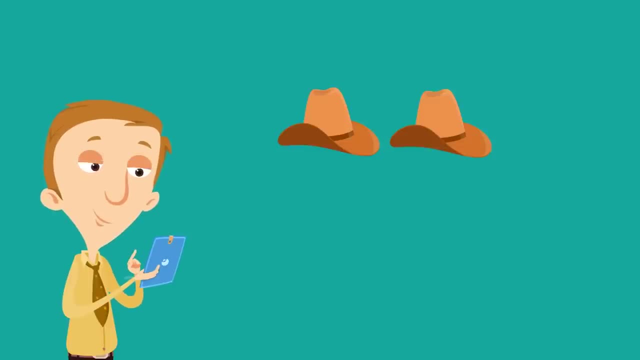 Just when I get to on the top of the bus. Subtraction is when you have nothing and only one contact or number as a friend, And that's when you feel evenear when something's wrong, because someone has a friend And they're like buddies. 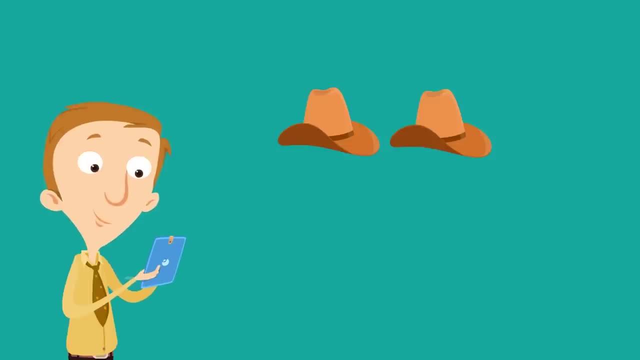 And they're like a pair of friends. and then Chomsky came by and I said: Oh, I'm going to have to do subtraction again. I'm going to have to subtract again. old Chomsky, You know that, Choms. 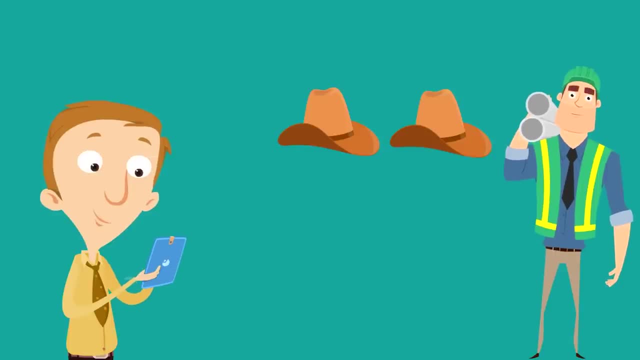 He came by I said I'm going to have to subtract again, I'm going to have to subtract one more. We lost our. because We lost our, We lost our color time. so I have two hats minus one, two minus one. so we subtract that one. we. 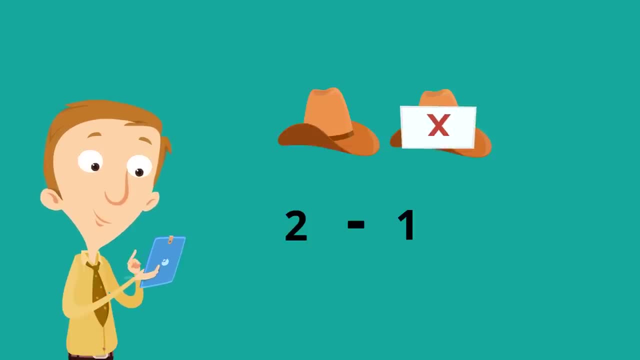 take that one away, and how many hats are left? what is two minus one? yep, two minus one equals one. there's only one hat left, which is fine. I mean, you know, I can only wear one hat at a time, and it was the same exact hat. I. 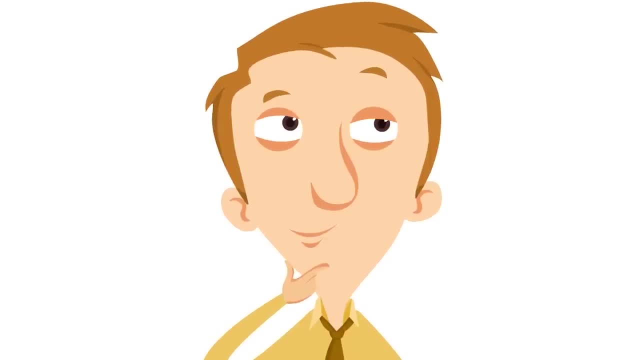 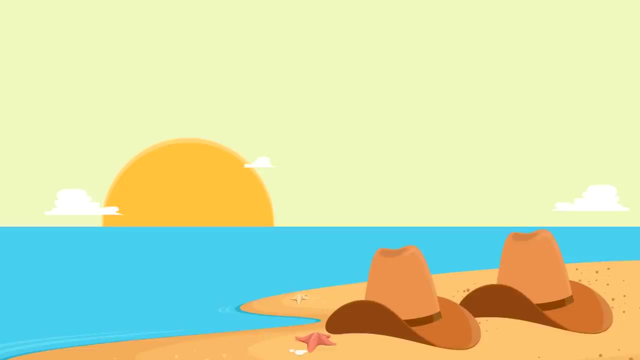 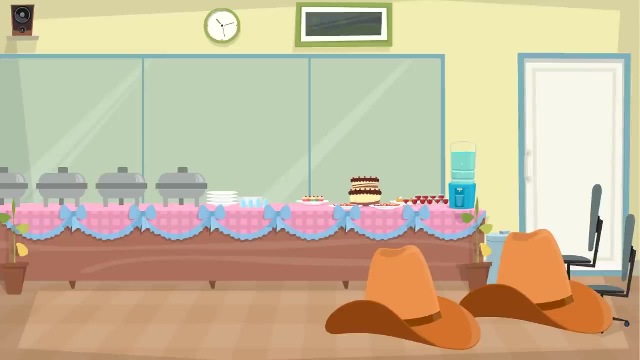 think about it. subtraction has been good. to me it's good subtraction is taking numbers away. sometimes I do wonder what would have happened if I didn't give that hat away. if Hattie still had his friend, they could have gone to the beach together, they could have gone to birthday parties together. but actually 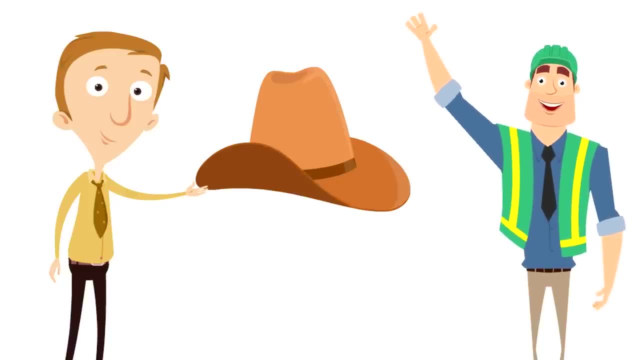 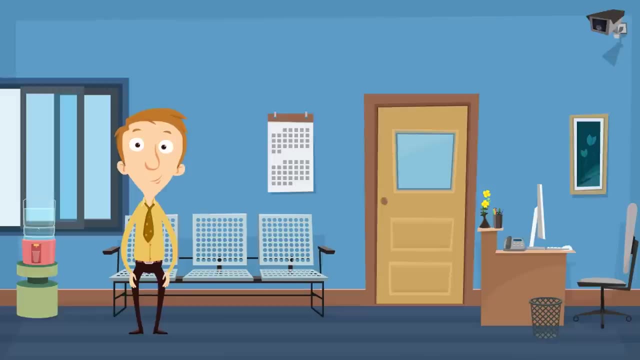 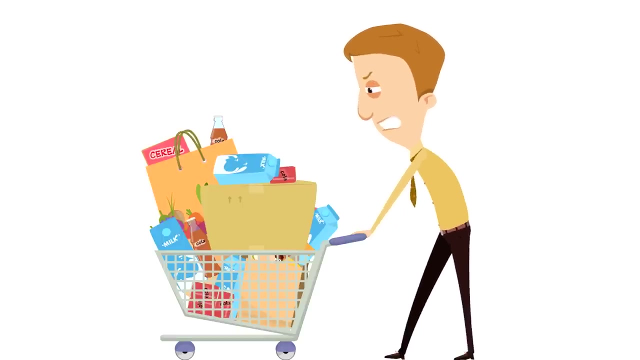 the hat had a better purpose- to make a friend happy. so in this waiting room, all I gotta say is thanks, subtraction, you are pretty awesome. oh, this is such a heavy cart. oh, my goodness, oh, oh, it's hard work. you know, a lot of times learning can be hard work too, but we hope that these videos are 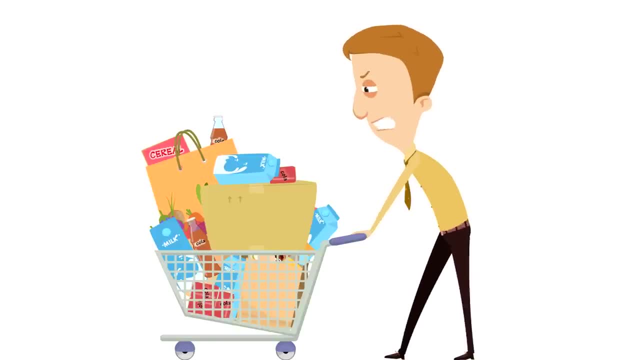 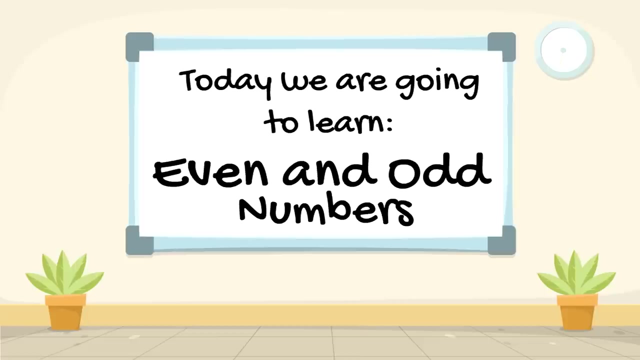 really helpful. make learning fun, so that learning isn't hard like pushing this cart. oh my goodness. all right, what's the next thing we should learn about? let's learn about even and odd numbers. a number belongs to one of two groups: either it's an even number or its an odd number. so what's going on? why is this even a thing? we're 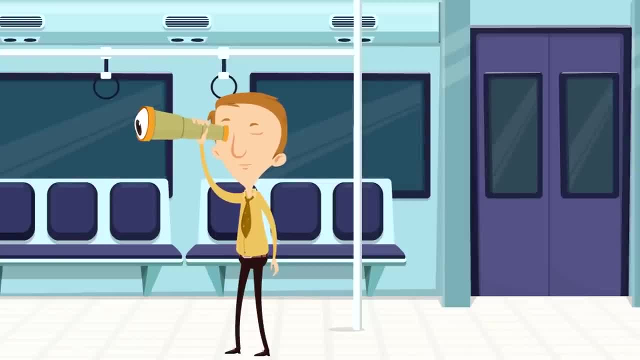 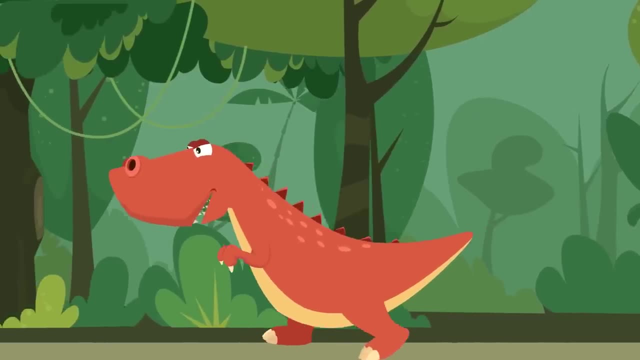 gonna talk about it. even an odd is actually pretty easy, but it's just a matter of knowing what to look for. so we're going to be like detectives together. okay, you're gonna have to have an eagle eye To help us out on our quest. We're gonna use dinosaurs. dinosaurs are awesome. 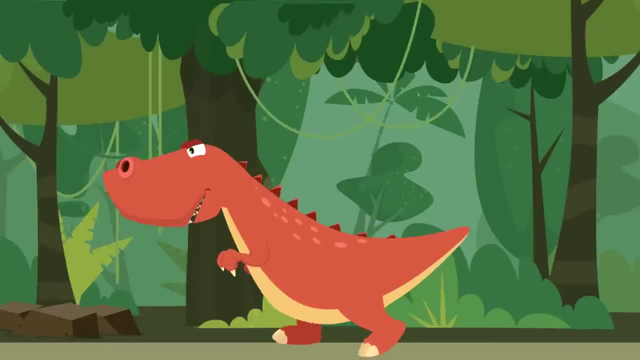 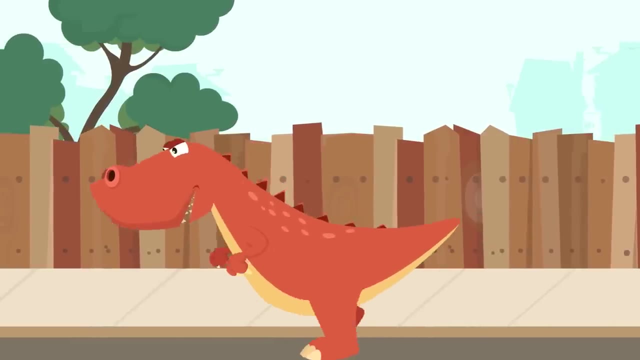 Here's a red dinosaur, That's. I don't know why it's windy, There's wind going on and I don't know What's what's. let's change the scenery, Let's let's make it more modern day. There you go. Look at that just walking through the neighborhood strolling. He's ready to help us. 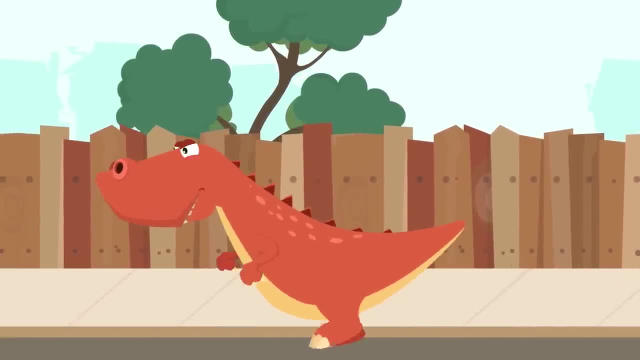 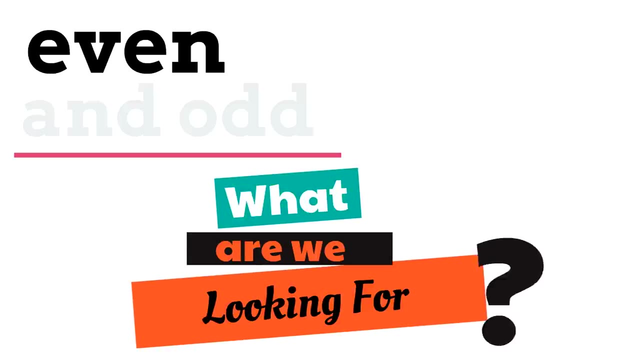 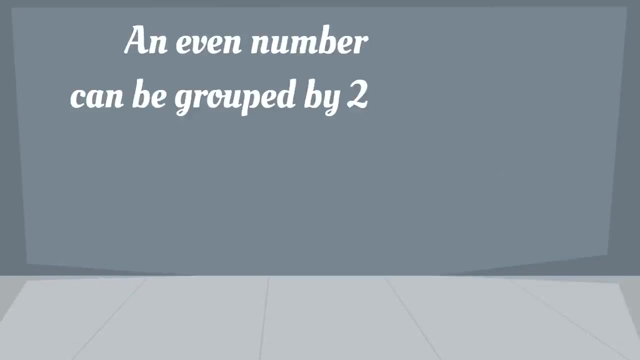 discover the secret Right to knowing even an odd. So what is this key that we're looking for? what are we looking for that will tell us if a number is even or if the number is odd? and Even number can be grouped by two. an odd number cannot be evenly grouped by. 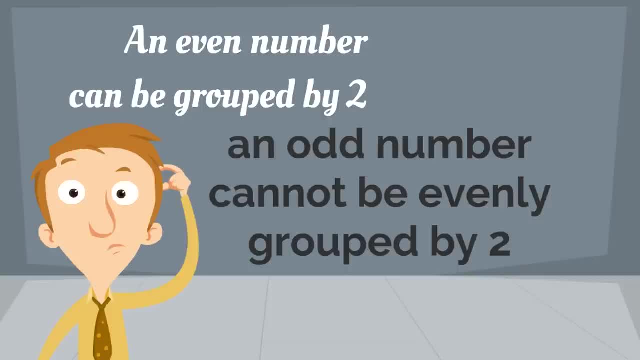 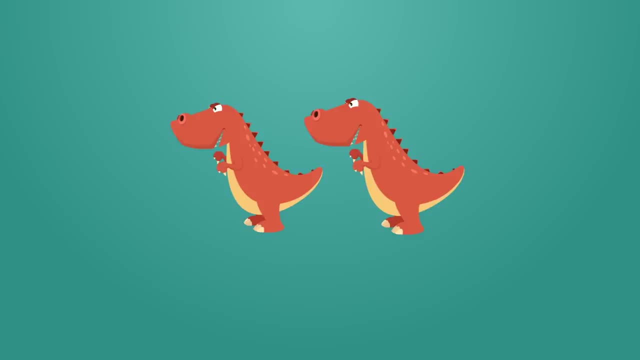 Two. so it's all about the number two, and that might sound confusing. Let me show you and you'll see, Here is the easiest number to do. We're looking for the number Two. okay, can it be put in a group of two? Well, yes, cuz it's the number two. We've got two dinosaurs. that makes two even. 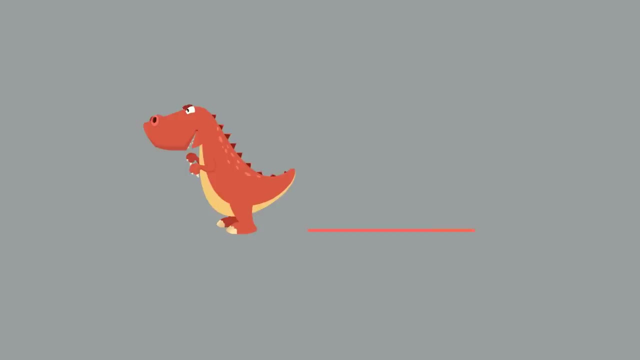 Now, this is odd. this dinosaurs all alone. He's not in a group of two. this makes the number one an odd number because he's all alone. That's odd. It's an odd number. Let's look back at the number two. see what's neat about this is it's an even group. 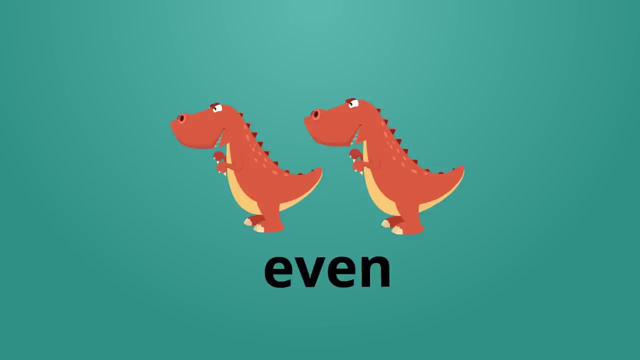 Of two. that means our dinosaur has a friend, he can talk to his friend, He can hang out. It's not. it's not weird, It's not odd, It's an even number. Here we have three dinosaurs. now Can we put the number three in even groups of two? well, 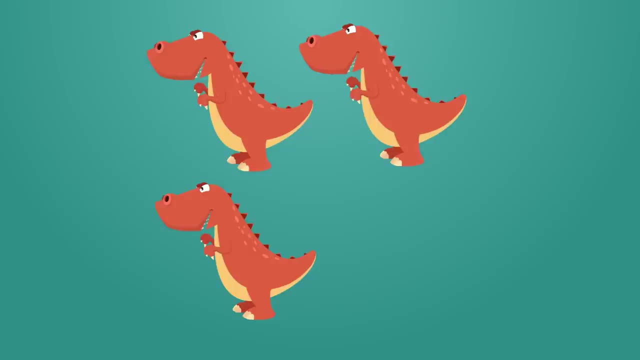 No, because that third dinosaurs, all alone, the top two dinosaurs, have somebody. three is odd. There's one that's missing a partner. Here we have four dinosaurs. now We're looking for groups of the numbers. number two: Now we have two groups of two here. That means it's an even number Each. 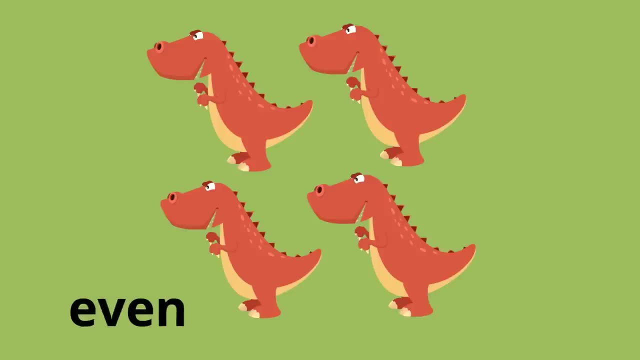 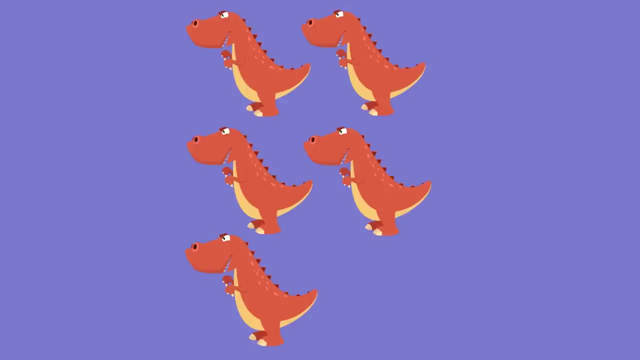 dinosaur has a friend. Wow, five dinosaurs. But look, one on the bottom doesn't have a pal, doesn't have a friend. That's odd. It's not evenly grouped into two. Five is an odd number. Hey, buddy. okay, don't run. Okay, we'll get back to the even numbers, I know. 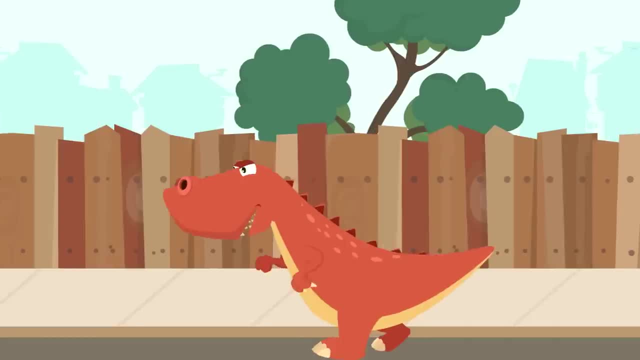 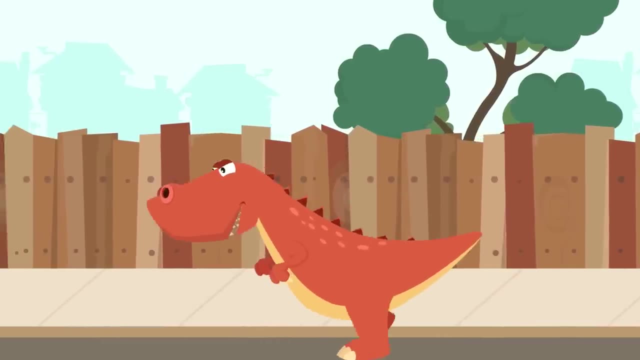 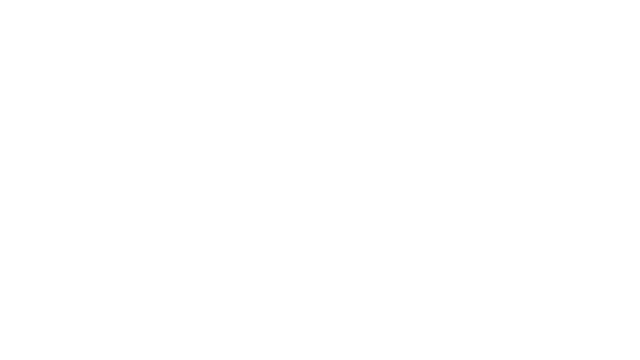 you don't like the odds, You don't like being the odd dinosaur out, It's okay. I promise this next number is going to be even, because it goes for even odd, even odd. Just hang on, Man dinosaurs, you know so temperamental I mean. what's that all about? I mean a dog. 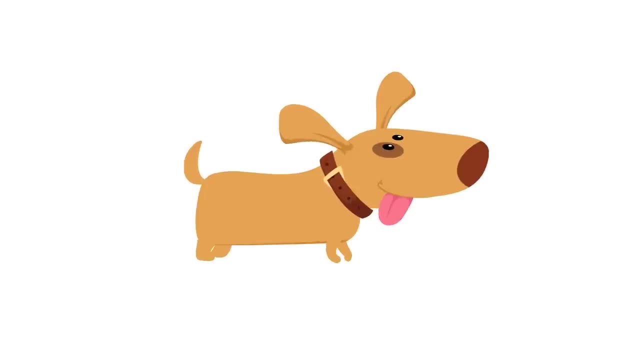 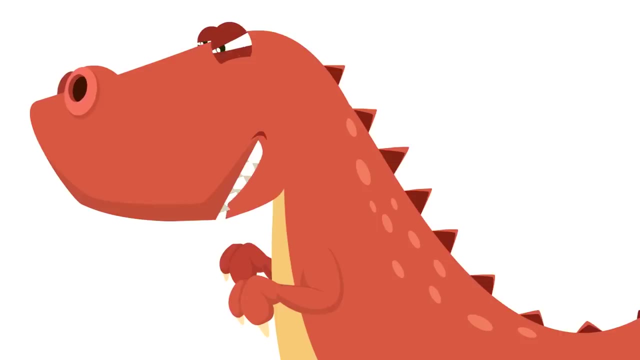 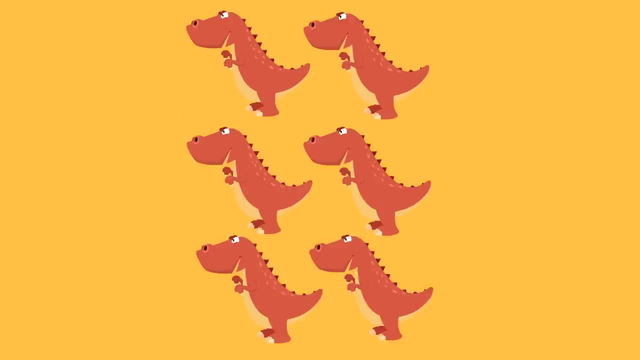 a dog wouldn't have done that. You know, dogs are better, I think now, than dinosaurs. you know, I'm just kidding. Dinosaurs are better than dinosaurs. Dinosaurs are so cool. Moving on Here, we have six dinosaurs Now. each dinosaur has. 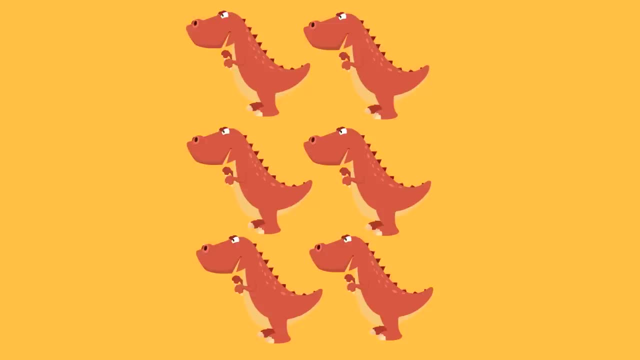 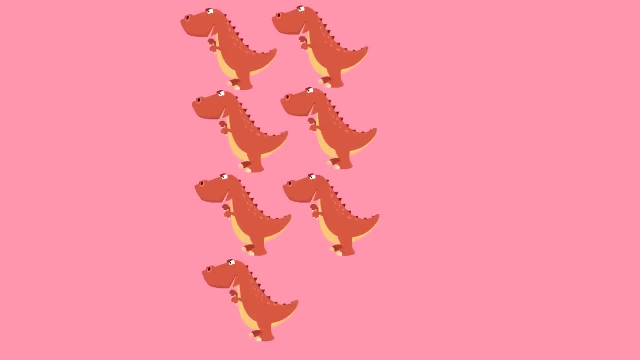 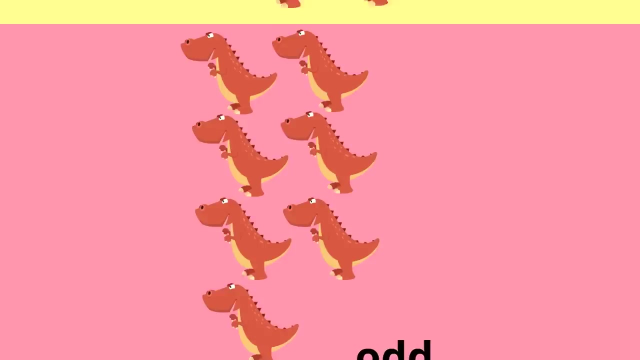 a friend. That means six is even. You can split it up in groups of two. Oh, here we have seven dinosaurs, but there's one dinosaur that's all alone. Six of them have friends. one is all alone, doesn't have a pair. Seven is odd. The number eight Does everyone have. 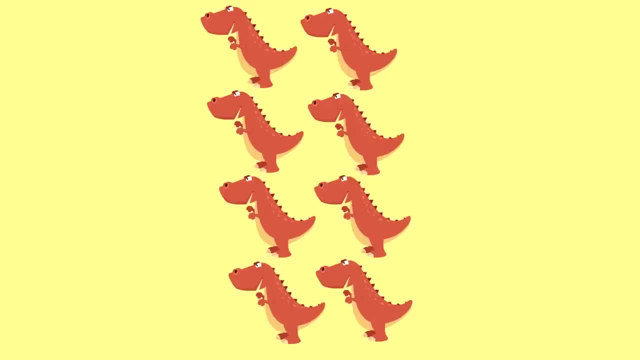 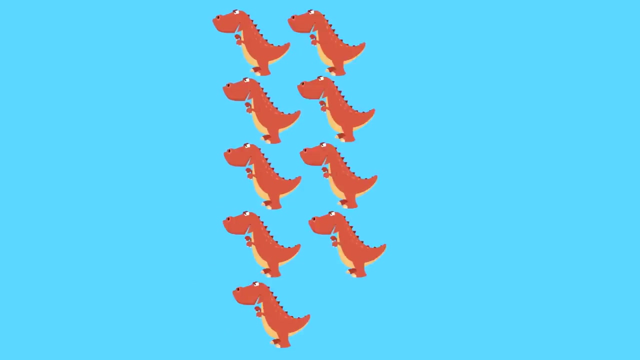 a friend. Yes, There's no one without a friend. Number eight is an even number. It splits up into two very nicely. Eight is even. Let's go even higher. The number nine. Now you can see really quick, it's easy to spot: Is nine even or odd. Nine is odd, Nine is odd. 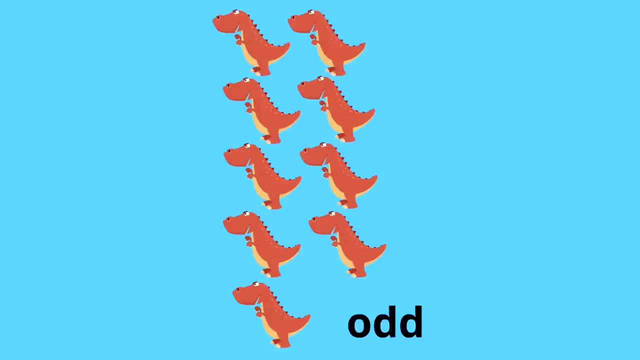 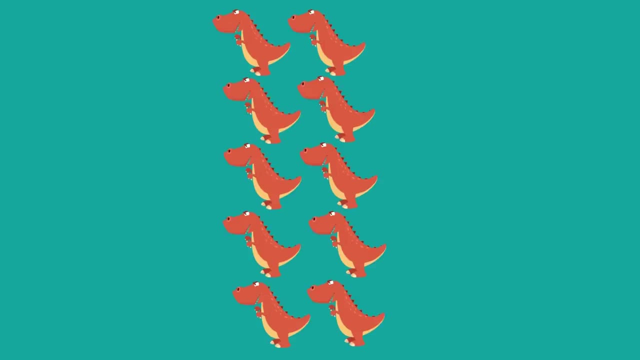 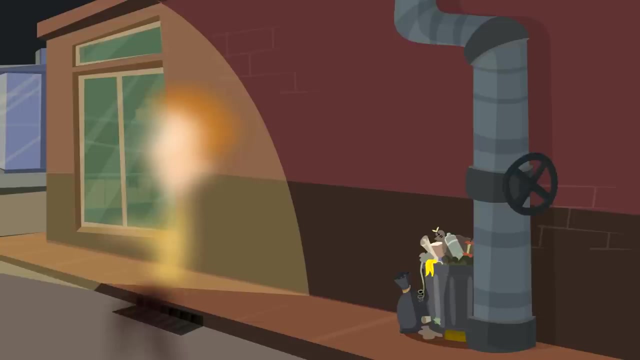 is odd. Oh my goodness, Ten. Ten Is it even, or is it odd? You tell me, You know how to do it. Now you know the trick. Yes, ten is even. Everybody has a friend. Now we're. 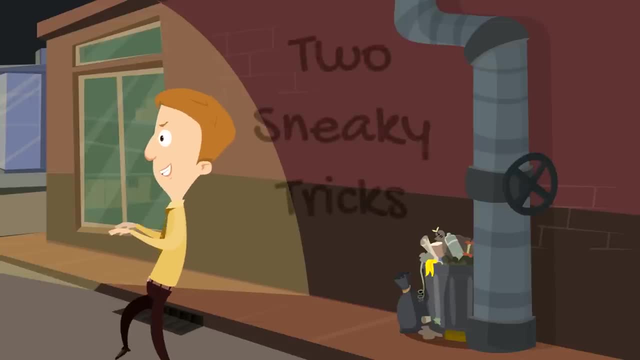 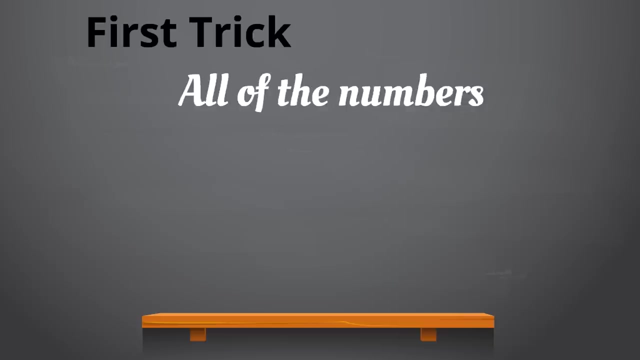 about to teach you two sneaky tricks that you can use with even and odd numbers. You okay. so seriously, it's well, it's not. it's not really sneaky anyway. so this first trick is that all of the numbers alternate from odd to even and back, and 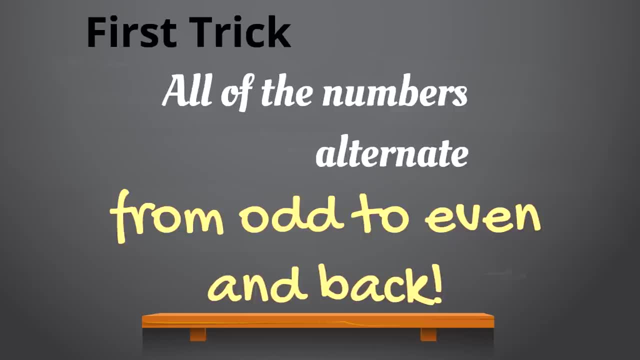 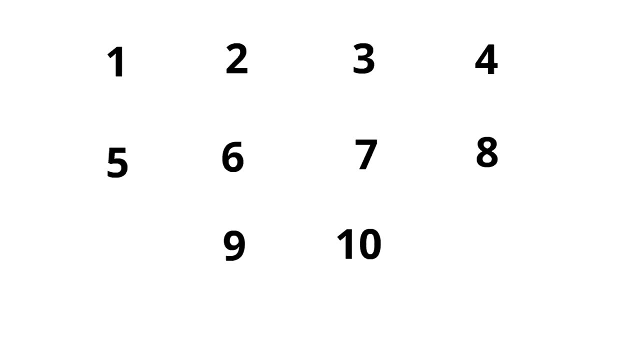 we're gonna show you what that means and what that looks like. here we have the first ten numbers, numbers one through ten, and the trick was: all of the numbers alternate from odd to even and back. do you remember if number one is odd or even? yes, number one is odd, because remember number one's all by himself. 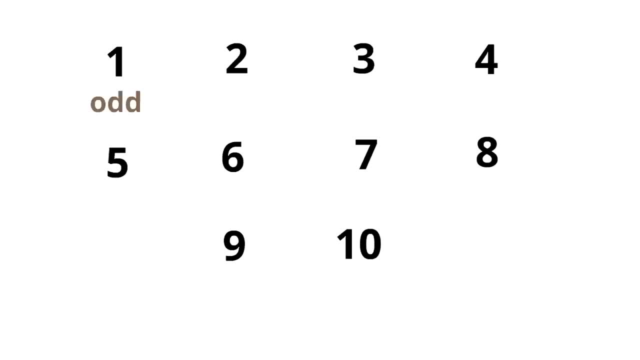 doesn't have a friend, doesn't have a partner. it's not an even number. number one is odd. now we remember number two, right, number two is even. yes, because it can be grouped in two, because it is two. now, if the number one is odd and the number two is even and the number one is odd, 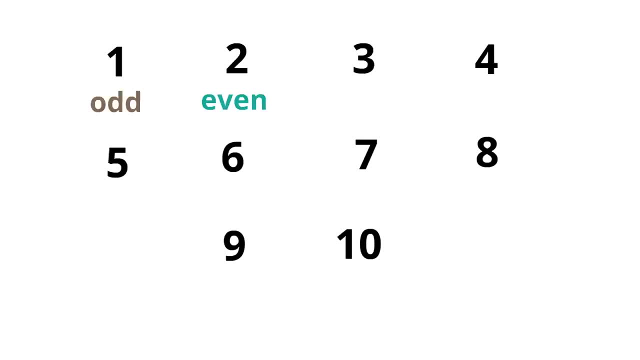 they alternate, that means which one is number three? it's odd. this is where it gets fun. if three is odd, then that means four is even good job. and if four is even, that means five must be odd, yeah. and if five is odd, that means six must be- you guessed it- even. and if six is even, that means seven must be odd. 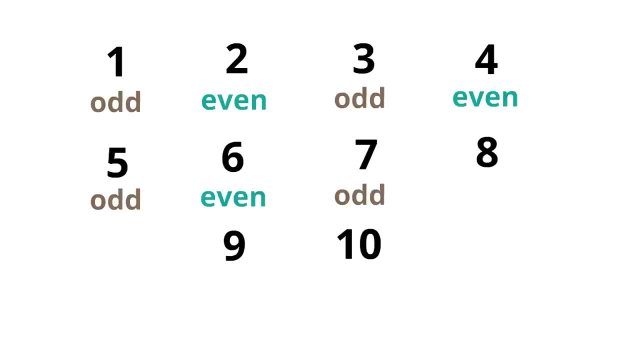 yes, seven is odd. if seven is odd, that means eight is. come on, what's the pattern? eight is even, and if eight is even, that means nine must be odd and nine is odd. come on, is this not just the most fun trick ever, ever? if 9 is odd, that means 10 is even. they all alternate. so the first trick is: 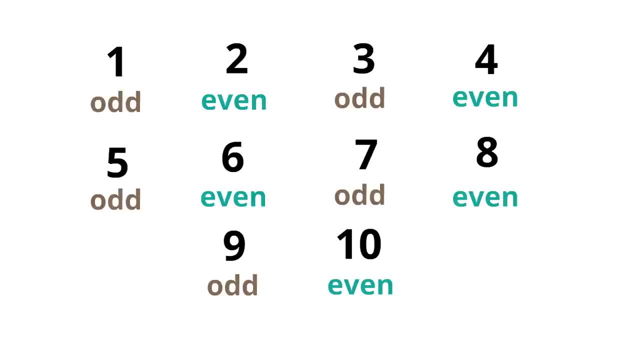 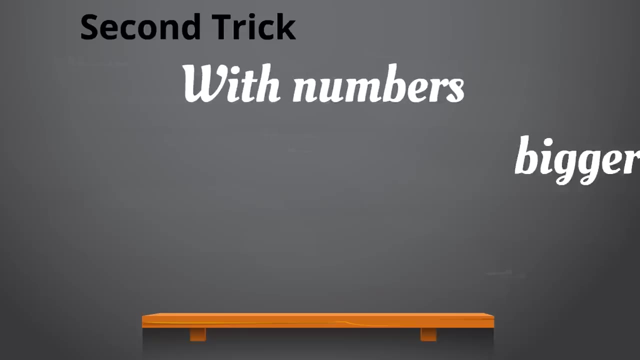 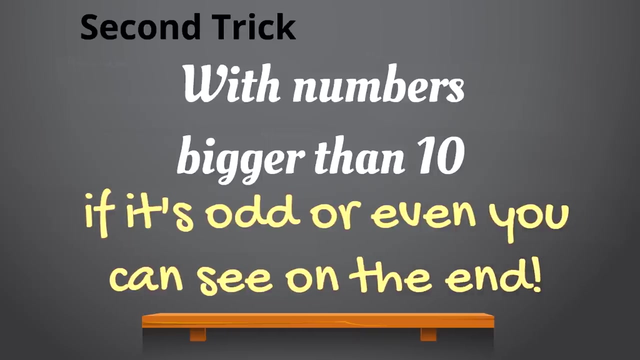 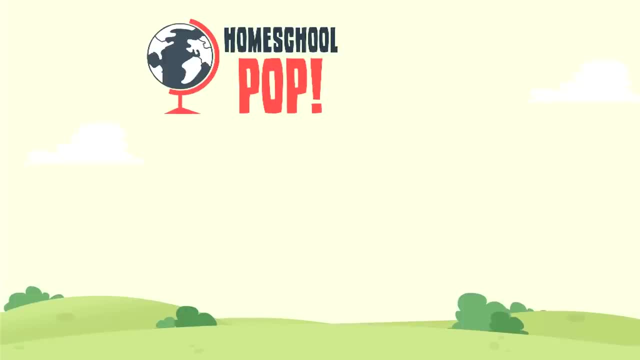 demonstrate. let's play a game. we here at homeschool pop call odd or even. we're gonna look at a number that's bigger than 10. we're gonna look on the end to see if it's even or if it's odd. our first one is the number 21. is it odd or is it even? it's odd? how, why, what? 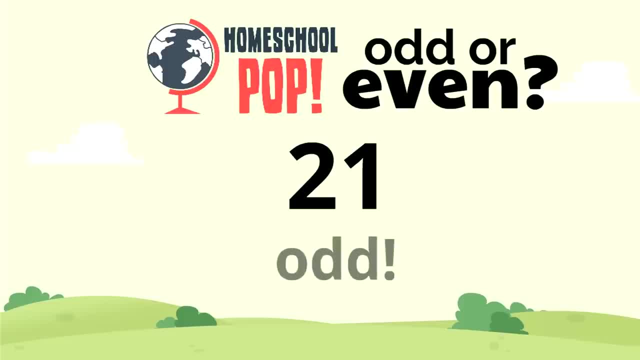 we look on the end, the end is a 1. 1 is odd. it's all by itself a 1 is odd. so 21 is odd because 1 is the ending. did you know that means 71 is odd and 101 is odd and 131 is odd and the number 1001 is odd. why they all end? 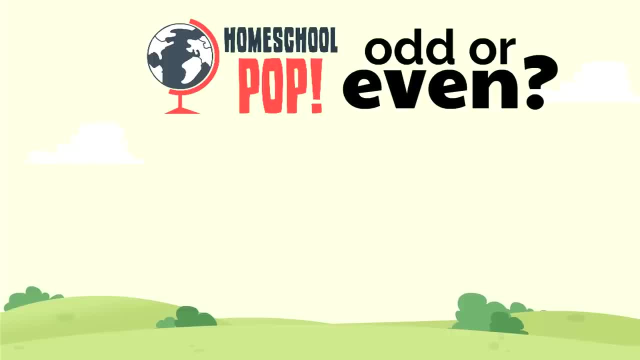 in one. let's try this one, the number 32. is it odd or is it even? 32 is even. well, how do we know? because of the ending. look at the ending. it's the number two. two is an even number because it's a group of two. it can be put in groups of. 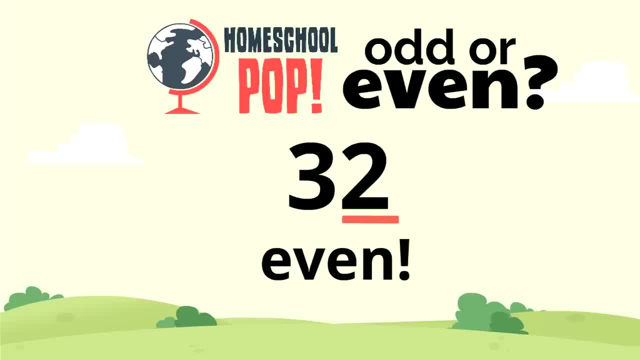 two because it is two. the same rule applies. this is the second trick- with numbers bigger than ten, if it's odd, or even you can see on the end, every single number that you can think of ends in two is an even number. let's try one. that's a. 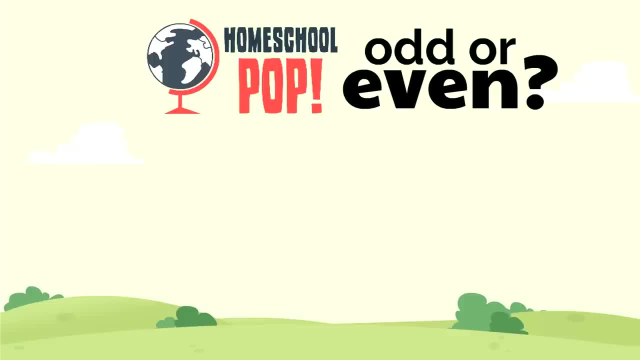 little more tricky. let's try the number: 100. is 100 odd or is it even? 100 is even, it's even and we know that because of the ending, it ends in a zero. now remember. second trick: with numbers bigger than 10, if it's odd, or even you. 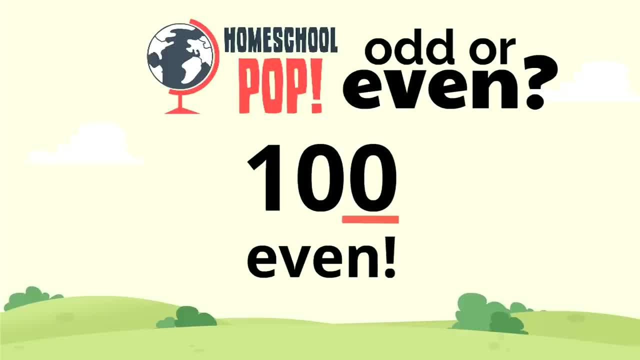 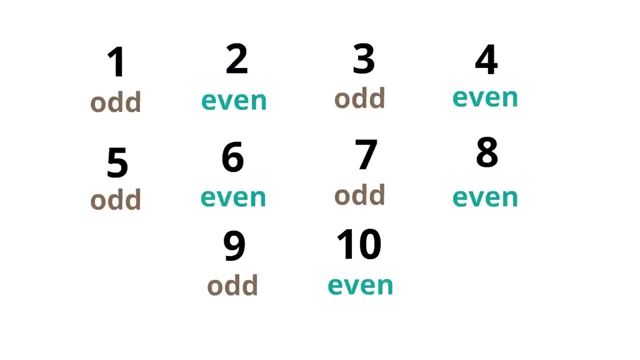 can see on the end and is a zero in. every number that ends zero is even. let's look at the chart again, as you can see: 10 on the bottom ends in zero and its even. every single number that ends in the zero is even, just like every number that ends in a one is odd. 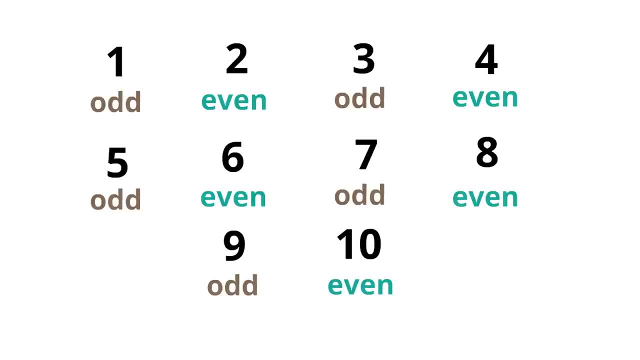 every number that ends in the two is even. every number that ends in a three is odd, because three is odd. every number that ends in a four is even, and it goes on and on. numbers that end in five are odd, numbers that end in six are even. numbers that end in seven are 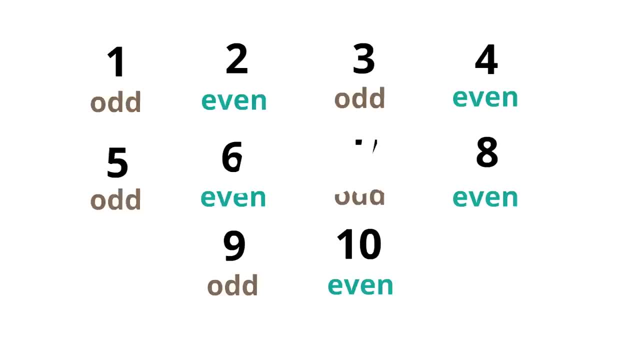 odd. numbers that end in eight are even, numbers that end in nine are odd, and then numbers like ten end in zero are always even. so there you go: odd and even. as long as you learn these, you'll know any number, because the endings always tell you if it's odd or even. so, once you know these, you'll know all of them. 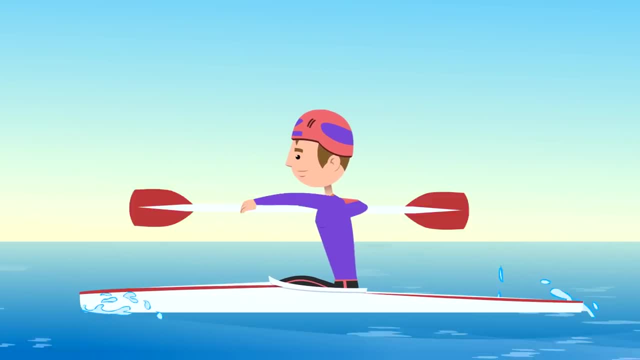 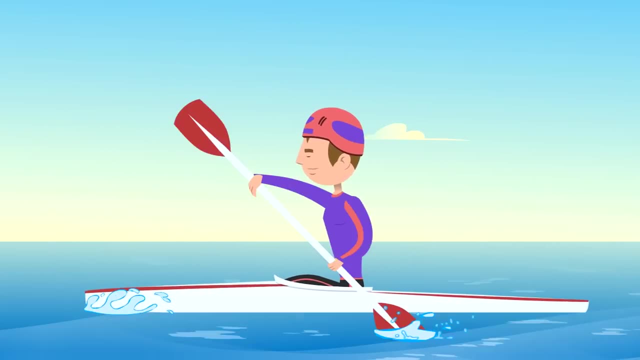 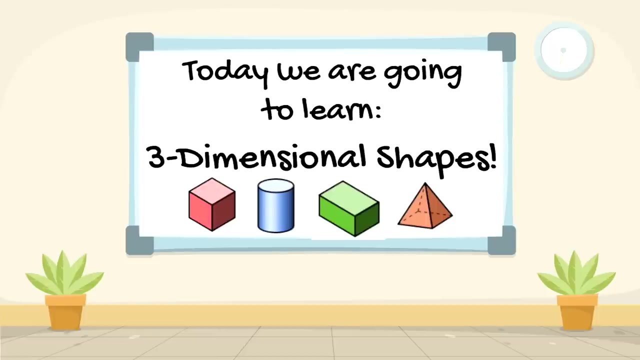 you're doing great. you're increasing your skills, just like this racer. you know racing on the water. you're increasing your skills. you're doing a wonderful job. and next we are going to learn about three-dimensional shapes. this is gonna be awesome. love the 3d shapes a lot of. 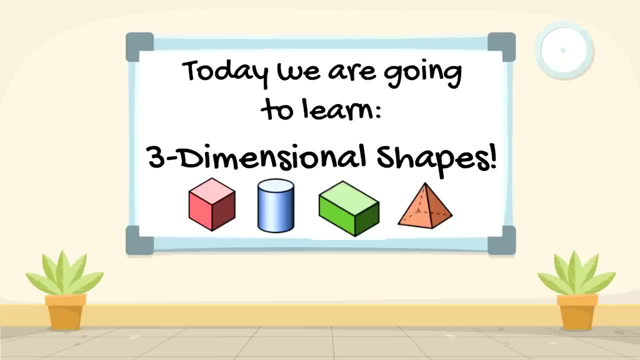 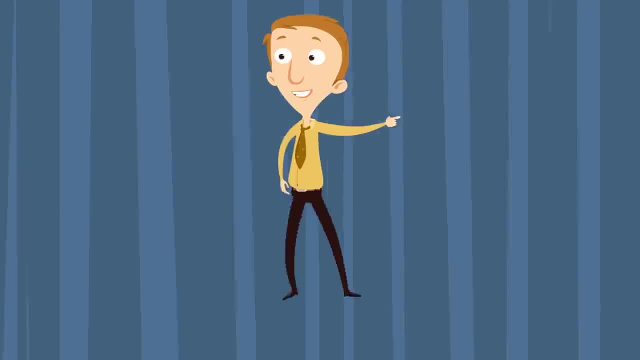 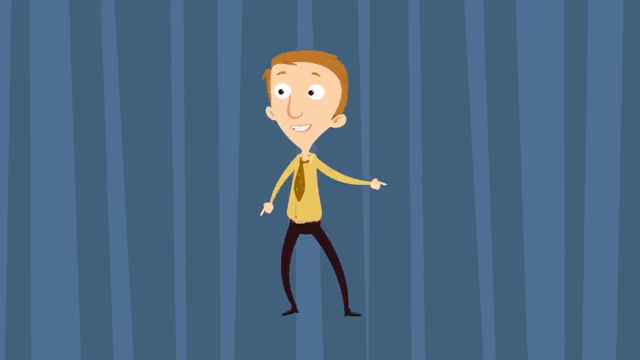 people know the 2d shapes. you might not know the 3d shapes. you're in the right place. before we get started, just dance here real quick. this is really cool music. I really like this. I like the dance. you know some people- they're not dancers- I dance, I dabble and dancing. 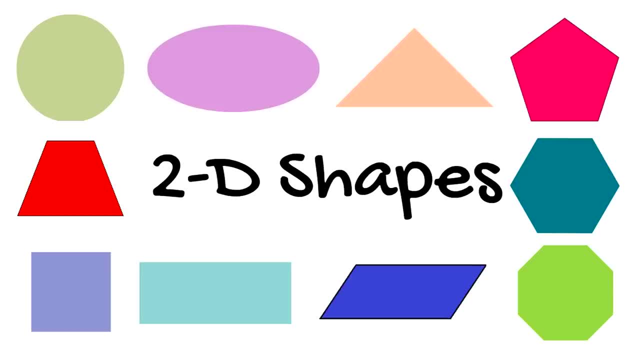 you know dance, I dabble and dancing. you know. All right, That's enough. Can somebody turn that music off? Seriously, I can't teach like this. I can't teach with this music going on. I feel like I'm in a candy shop. Let's just turn the music off, please. Thanks, 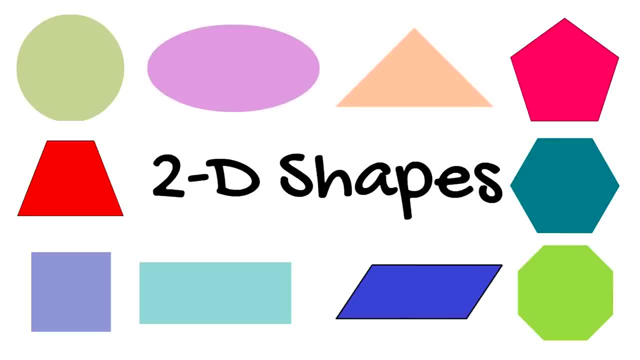 So here they are, our old friends, the 2D shapes. You're familiar with these, You know you're familiar with the circle, the oval, the triangle, the pentagon, the trapezoid, the hexagon, the square, the rectangle, the parallelogram and the octagon. 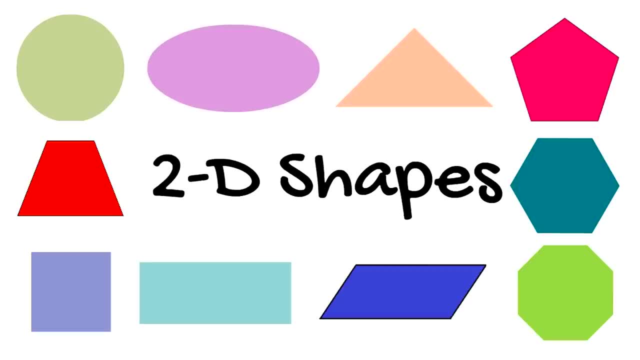 And these aren't all our shapes, our 2D shapes, you know, but these are all family friends of ours. We don't want to just forget about these And before we look at 3D shapes, it's really important for us to look at these shapes again, because these are our old friends. 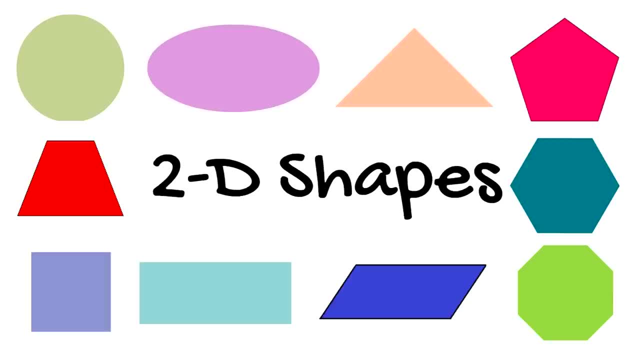 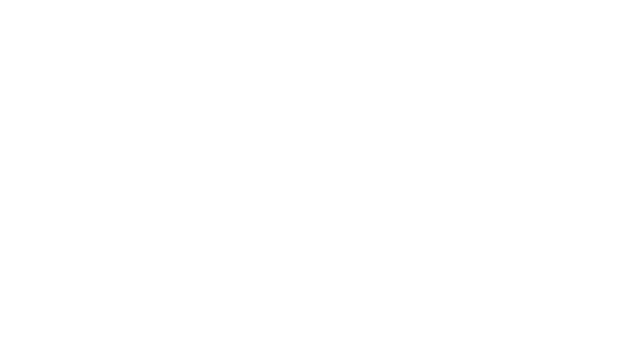 So we're going to look at each one of these one by one, just to make sure you know who they are before we learn all these new shapes. This first shape doesn't even need an introduction: It's the circle. the circle, that round figure. It's awesome. We love this shape. It's one of the first ones we ever learn: the circle. 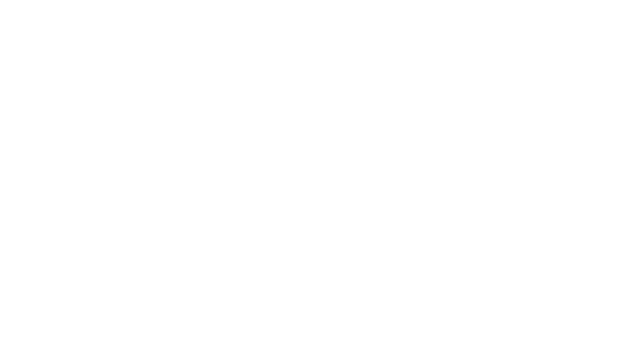 This next shape is one of the stretchy shapes: the oval. It's like a circle got stretched out, It's elongated. It's a tremendous shape, the oval. Here's another familiar shape: the triangle. three sides. We love the triangle. The triangle is great. the three-sided friend. three sides, a triangle. 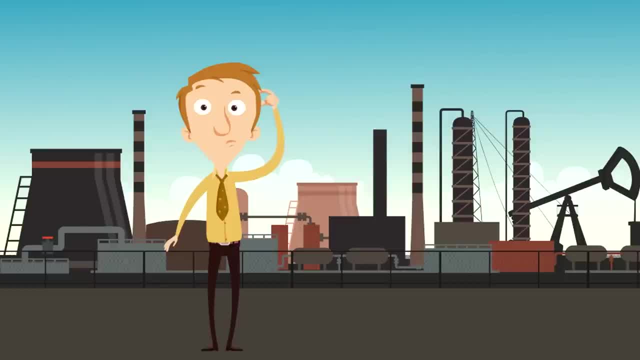 Here's another familiar shape: the triangle- three sides a triangle. Here's another familiar shape: the triangle- three sides a triangle. Wait, I keep saying we love the shapes. I mean we like the shapes, but do you love the shapes? Do I love the shapes? I mean, I don't know, Maybe I need to take it easy here. 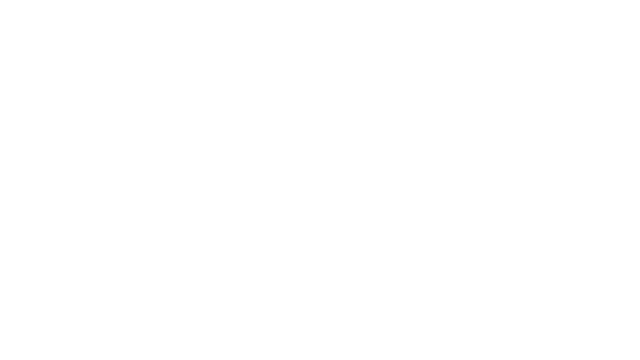 All right, let's keep going. Ah, the square, four sides all equal. You know, the square's good, The square's a good shape. you know, Sometimes you just need a square, Sometimes you just need, Sometimes you just need. 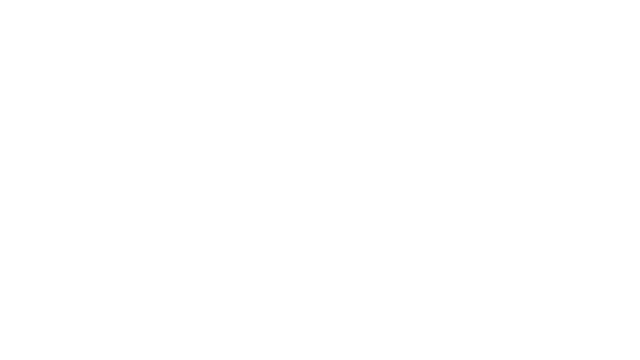 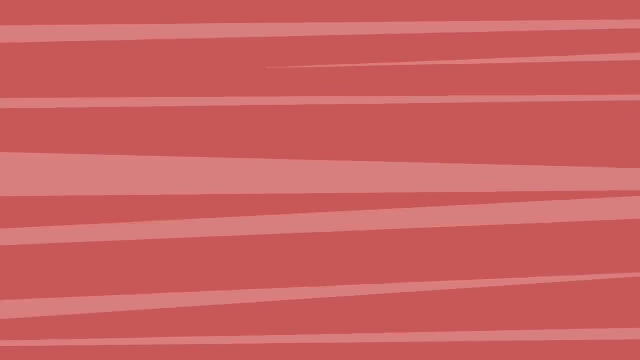 a square. Here's the rectangle. The rectangle is longer than the square because not all four sides are equal: The rectangle. I know, I know, I know We're in the middle of something here, but I have to share this again. So what do you call a hamster with a top hat? 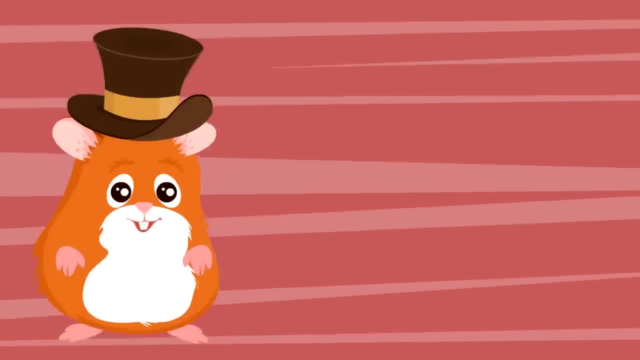 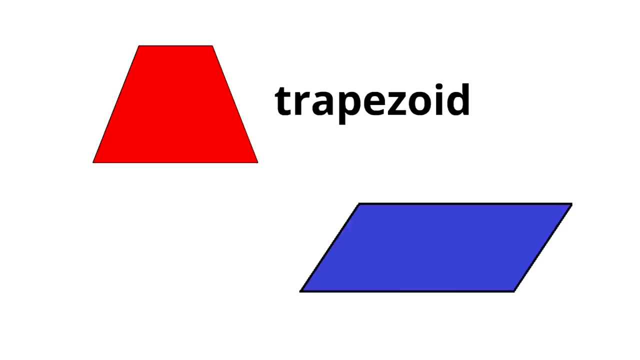 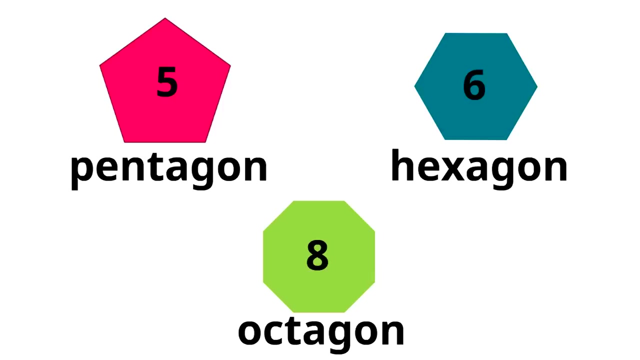 Abrahamster Lincoln- I digress- The trapezoid, a cool shape with two of the sides being parallel to each other. in the parallelogram, another four sided shape, Both pairs of sides are parallel to each other. And finally the pentagon with five sides, the hexagon with six sides and the octagon. 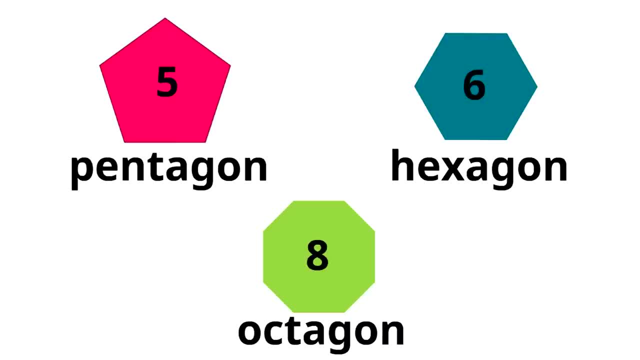 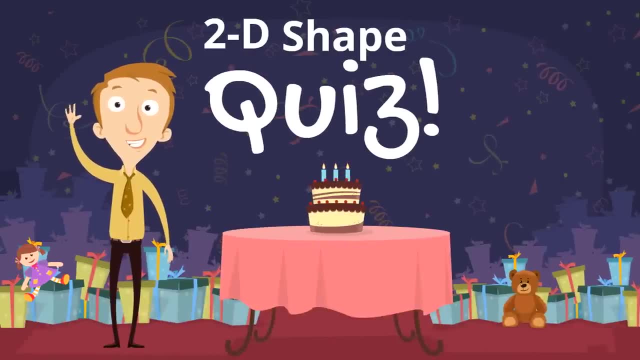 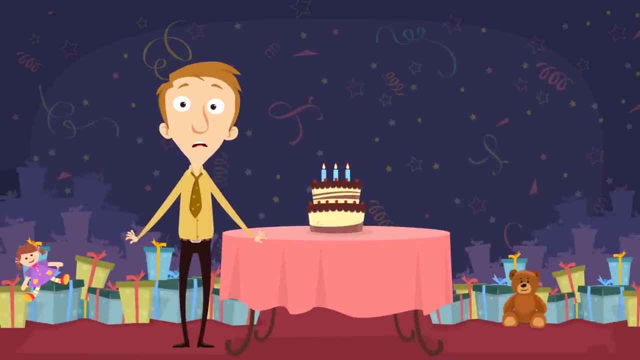 with eight sides. What awesome shapes. So let's go ahead and do a quick 2D shape quiz. I need your help. I want to see if you really learned these, if you really know these, before we get into the 3D shape. So help me out here. We're going to have an awesome time. Wait what? It's not my 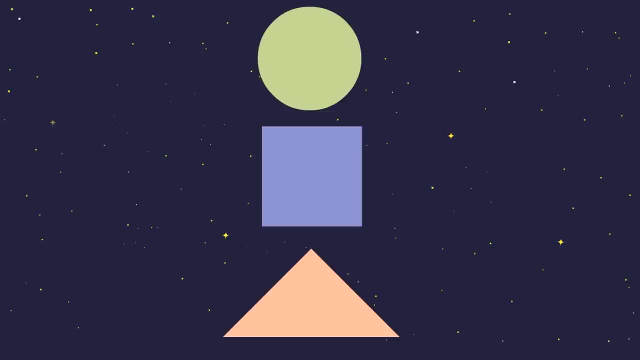 birthday. Oh well, What type of shapes do you have? What type of shapes do you have? What type is on the top? Yeah, a circle. What type of shape is in the middle? A square. Awesome, Okay Now. 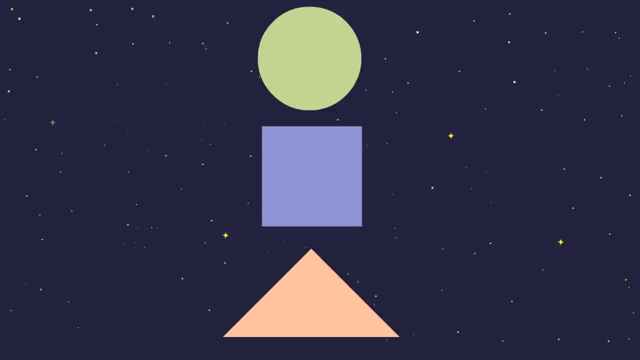 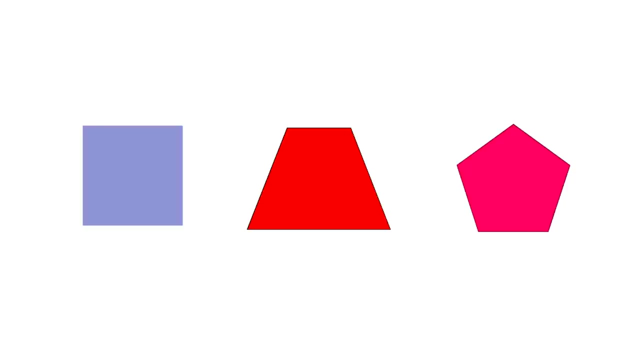 what shape is on the bottom? Of course, a triangle. Awesome job. Now we've got more. This is a little trickier. Which shape is in the middle? Yeah, a trapezoid. Which shape is on the right? The pentagon. Good job. And which shape is on the left? Yeah, the square. 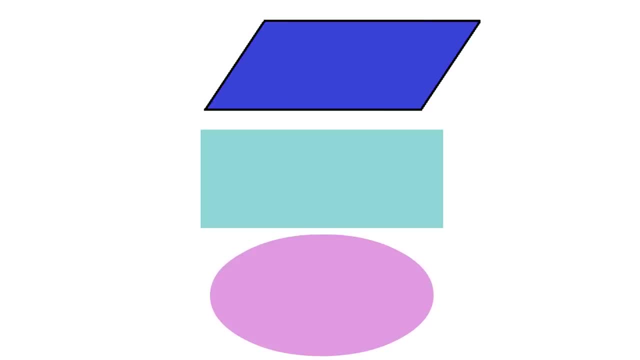 That's right Now. try these. Which shape is on the bottom? Yeah, the oval. Which shape is on the top? Yeah, the parallelogram. Which shape is in the middle? All right, The rectangle. great job. 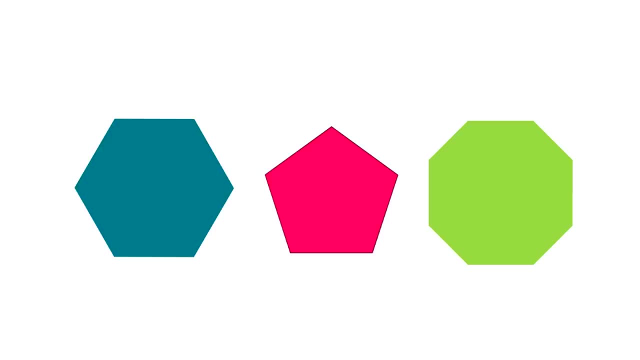 Oh my god, I don't think I can do this. I'm kind of nervous. I think I'm going to have a hard time. There you go, Okay, good job, Awesome. Now try some of these different shapes. which shape is on the bottom? Yeah, I. 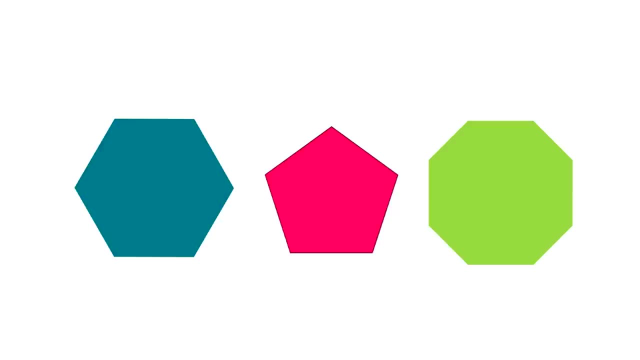 All right, the last one. Which shape is on the left? Yeah, the hexagon. Which shape is on the right? Great, the octagon. And which shape is in the middle? Phenomenal, the pentagon. All right, we're ready to learn the 3D shapes. 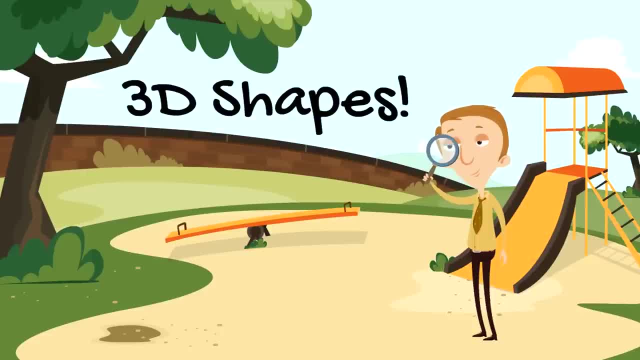 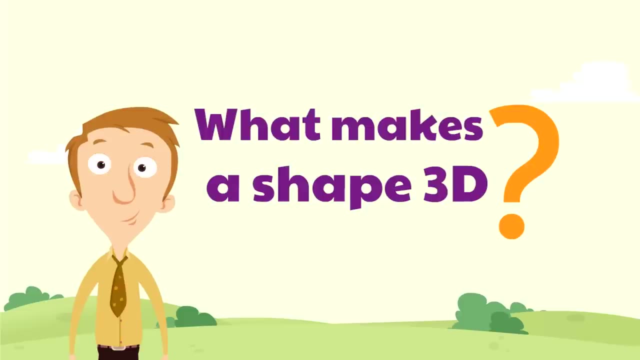 We're going to learn how to identify the three-dimensional shapes. If you struggled through the quiz, you might want to watch the first part of the video again. Otherwise, let's get started. So as we're starting out, it's important to remember what makes a 3D shape a 3D shape. 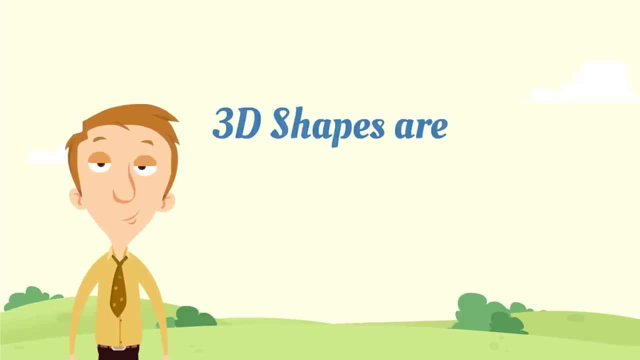 There's an old rhyme that says: 3D shapes are fat, not flat, And you can see that With the sphere, which is a 3D shape we're about to learn, and the circle, The circle is flat, but the sphere is 3D. 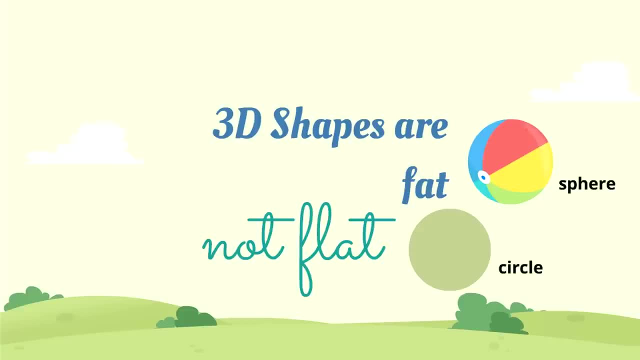 It's three-dimensional, All the shapes are like that, So let's learn all these 3D shapes. So the first 3D shape we're going to learn is the sphere, The one that we just mentioned. the sphere is the 3D version of the circle. 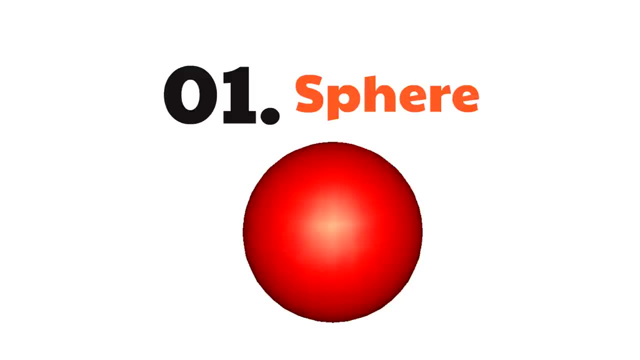 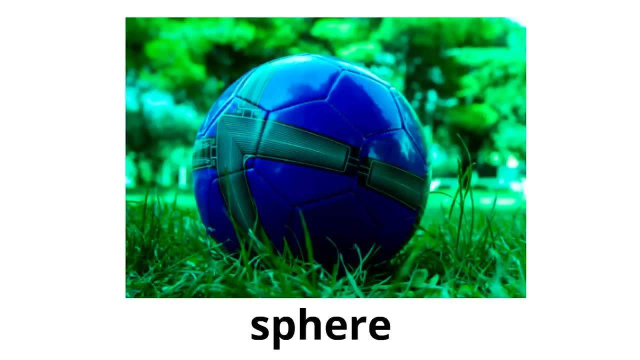 It's perfectly round. There are spheres all around us. One of the spheres we see all the time are balls like this soccer ball. A soccer ball is a sphere, It's perfectly round. It's a 3D circle. It's a sphere. 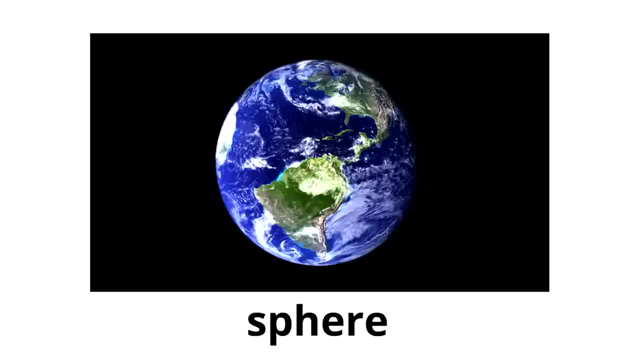 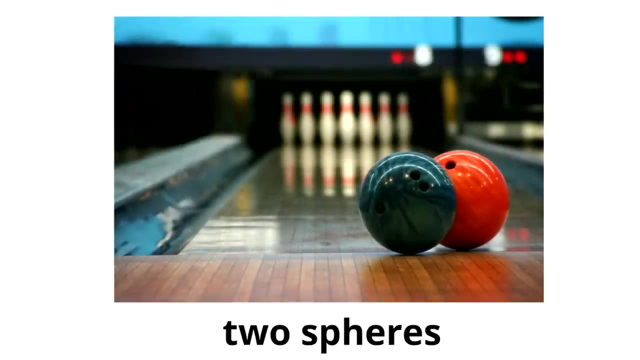 You know this sphere? Yes, it's the Earth. It's where we live. Our planet is a sphere. How cool is that? Our own planet is a sphere. Perfectly round, It's a sphere. In this picture, we have two spheres. 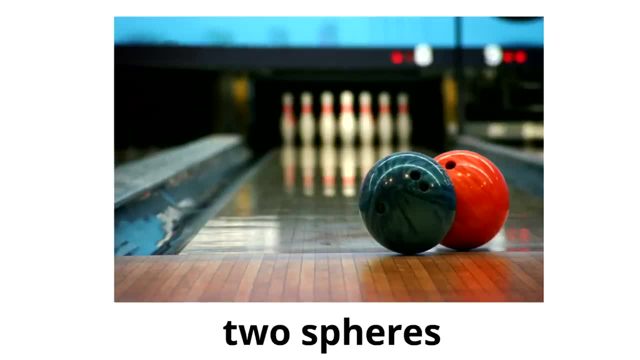 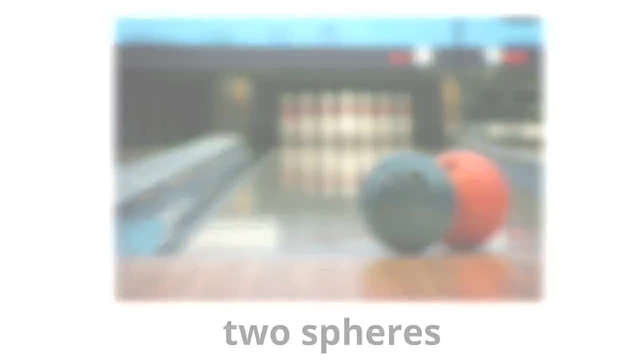 Can you spot them? Yeah, The two spheres are the two bowling balls. Perfect, round spheres. Spheres are all around us. Here we have a group of three spheres. You can count them right now: One, two, three spheres all together. 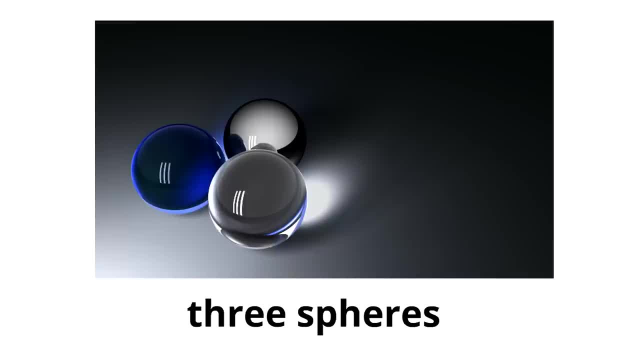 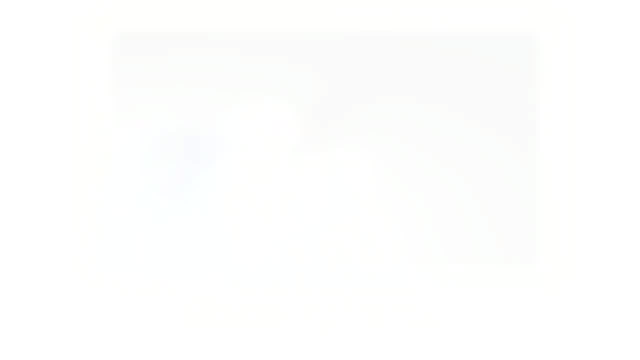 The shape of a ball, A sphere, Perfect round. sphere, Perfect round, sphere, Perfectly round. Not bad. There you have it, The sphere. What a cool 3D shape. to start with, It's round. There are examples all around us. 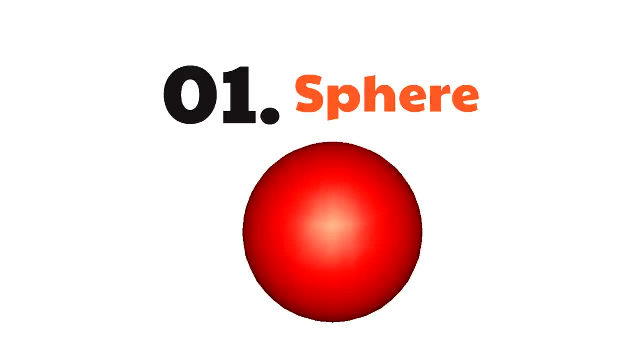 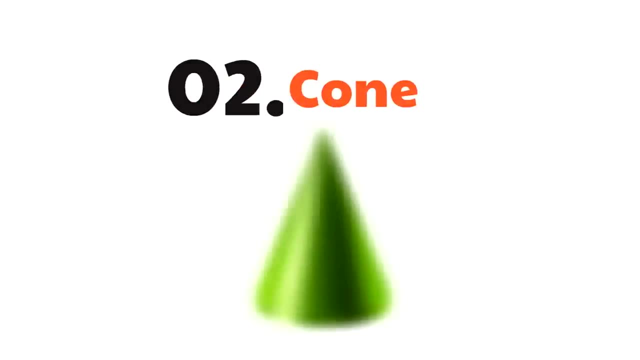 It's just so cool. You know what The 3D shapes are going to get even better. Our second 3D shape is the cone. The cone is a really cool shape with a circle as the base or the bottom, and it all comes up to one point called a vertex. 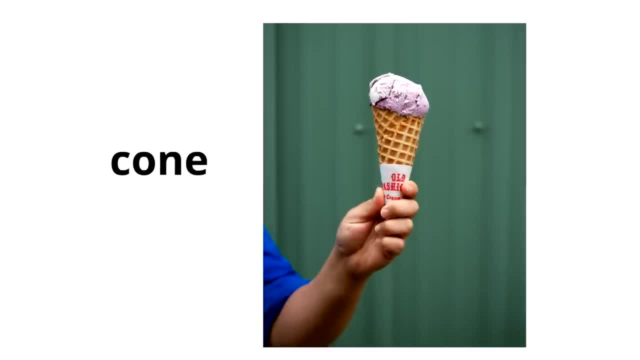 Here's an example of a cone. I think we all love the ice cream cone. If it doesn't have any ice cream inside and you flipped it upside down, you'd be able to see the circle base and it all comes up to one point called the vertex. 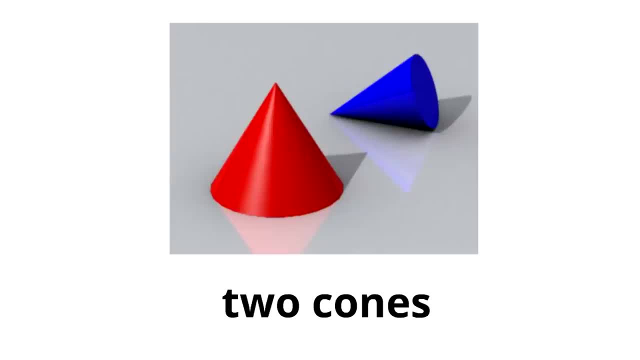 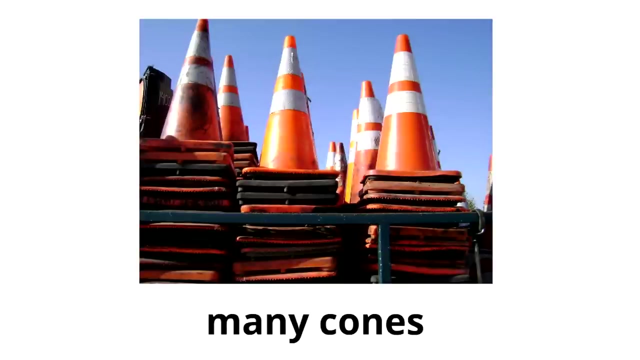 Here are two cones, a red cone and a blue cone, And you can see both cones have that circle base and it all comes up to a vertex. What wonderful cones. Have you seen these before? They're traffic cones. Here are many cones. I didn't count all of them, but there's a lot and they're wonderful, wonderful cones. 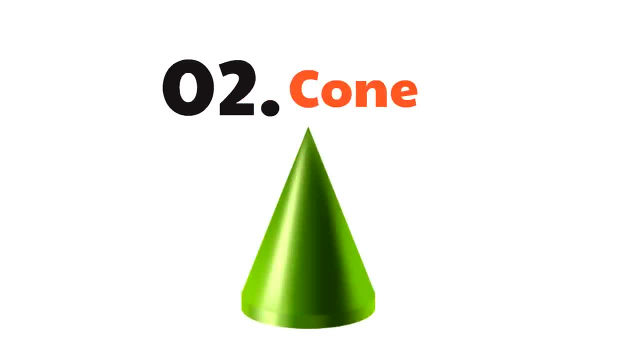 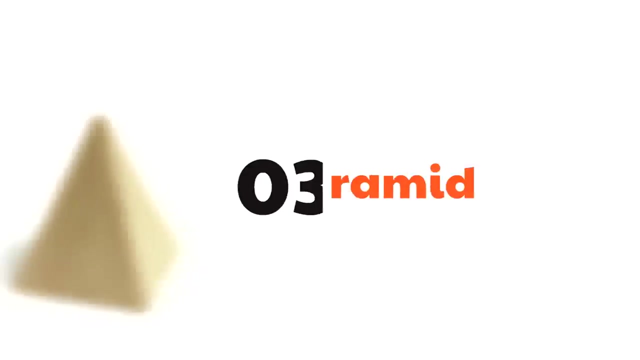 So that's our second 3D shape: the cone. A wonderful cone with a great circle base. It all comes up to one point called the vertex. How awesome is that? Our third 3D shape is the pyramid. I love the pyramid. The pyramid's great. 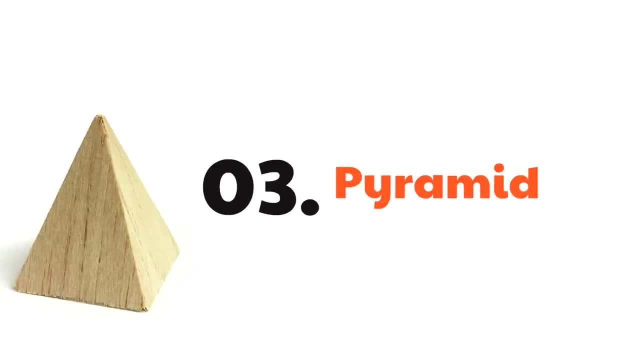 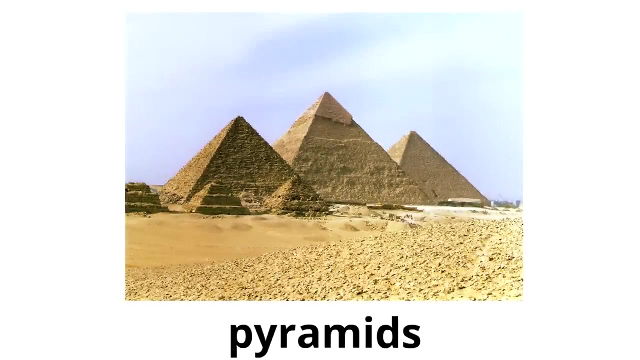 It comes up to one point: just like the cone, except the base is a square and the sides, instead of being smooth, they are triangles. Okay, like these are awesome. These are so cool. the pyramids of Egypt. You see that they have the triangle sides and the bottoms of these pyramids are. 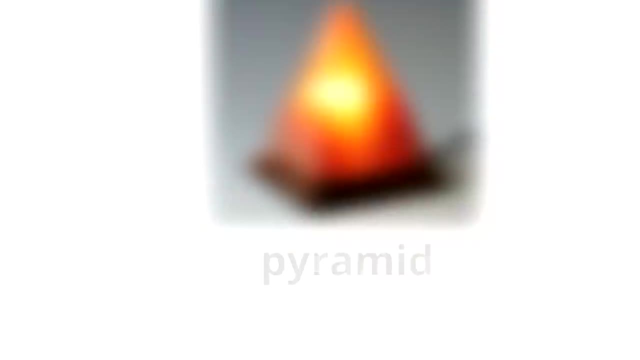 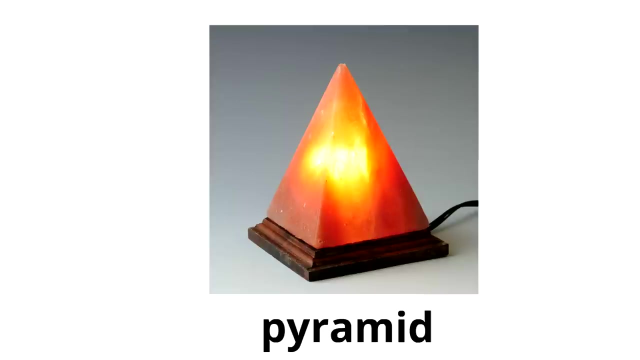 Square. they're awesome examples of the pyramid. This is a pretty cool pyramid. It's a decoration that you plug into the wall, But it's a great example of what a pyramid looks like. the bottom or the base is square And there's the triangles on the sides. How cool is this. 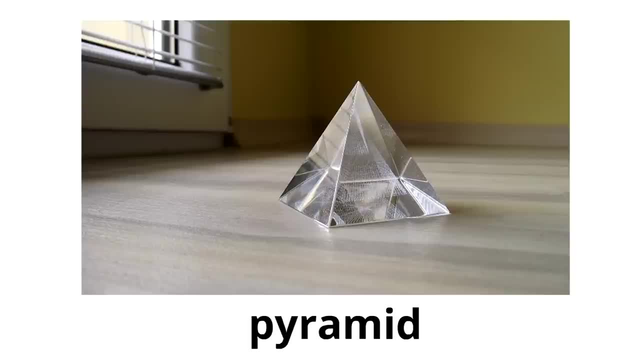 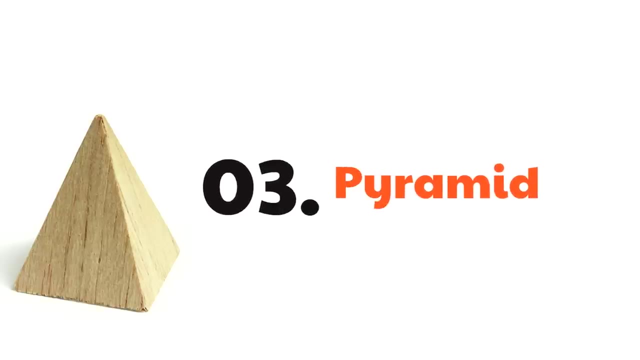 Here's another pyramid, and it's made of glass. There are so many decorations and things around, maybe even your house, that are shaped like a pyramid. because Pyramids look so cool, People love putting them everywhere. There you go. I mean, you know the pyramid, it's a good shape, you know you see a lot of them around. 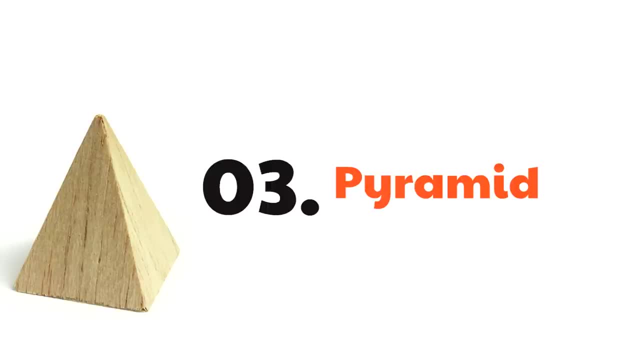 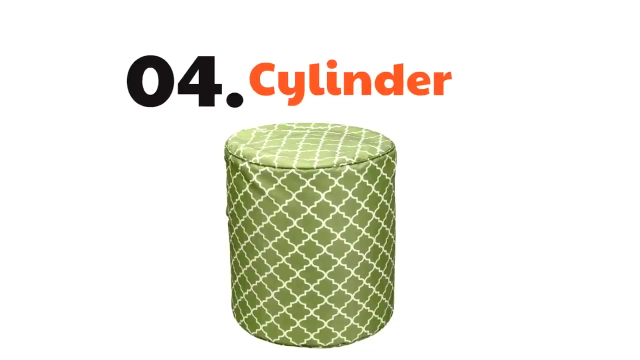 they've got the square bottom or base and the Triangles on the sides and all goes up to a vertex. It's a classic shape. It's pretty awesome. Our fourth, 3d shape is the cylinder. now, a cylinder is easy to spot because it's got a circle on the top and a circle on the bottom and it's 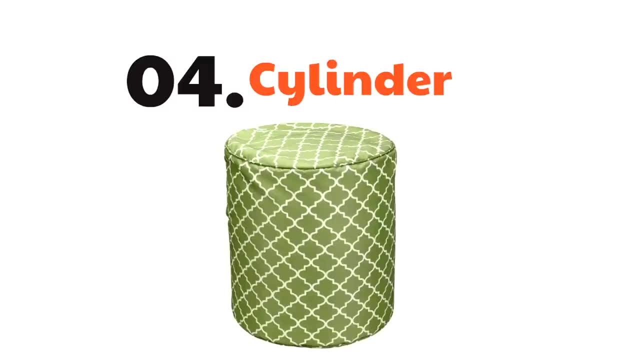 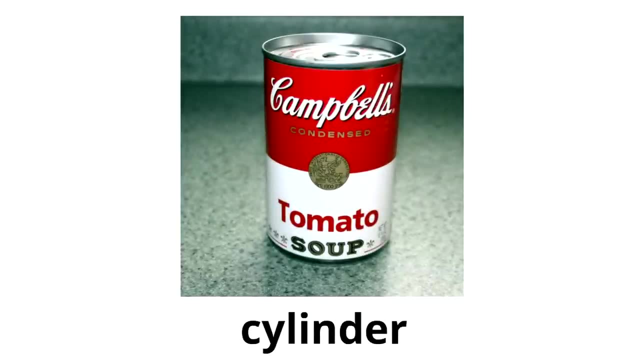 smooth all around. Here we have a can of soup and it's a cylinder. it has a circle on the top, a Circle on the bottom and it's smooth all Around. all cans and most jars are cylinders. Here we have three cylinders. They're candles and cats. 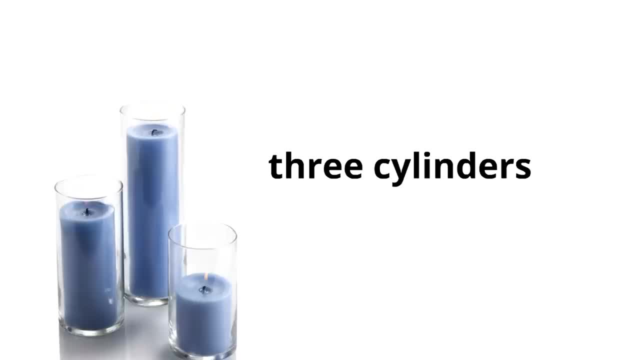 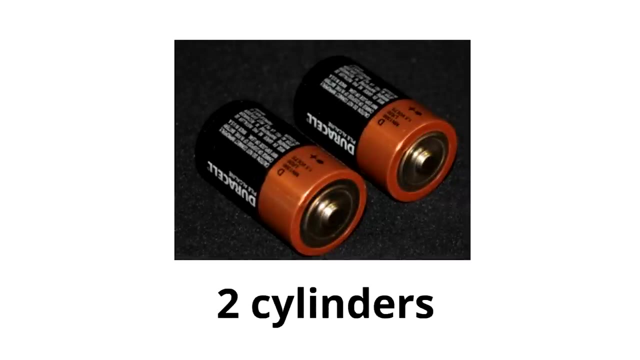 I'm telling you a secret: Most candles are cylinders. too right? This is just too crazy and too awesome. Here are two more cylinders. Are you kidding me? Are you kidding me? even batteries are cylinders. cylinders are seriously Everywhere: a circle on the top, a circle on the bottom and smooth all around. 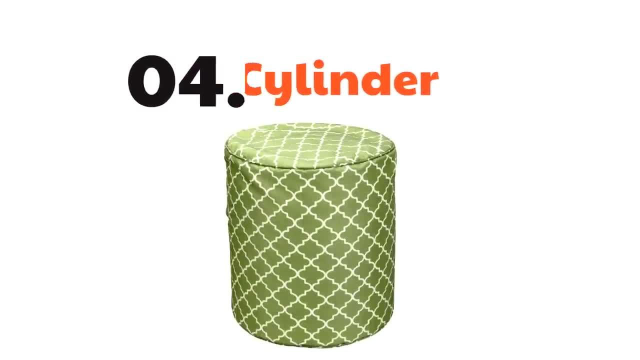 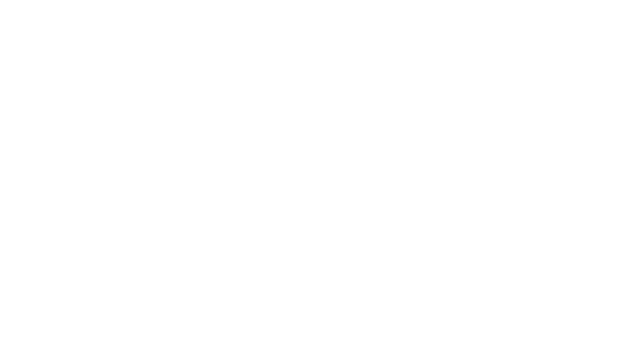 I mean really the cylinder is everywhere. I mean You know the circle on the top, circle on the bottom, smooth, all around cylinder. like what in the world do you have to be everywhere? okay, The next 3D shape is the cube. 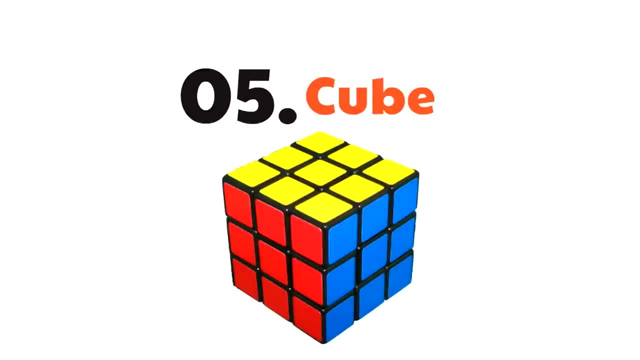 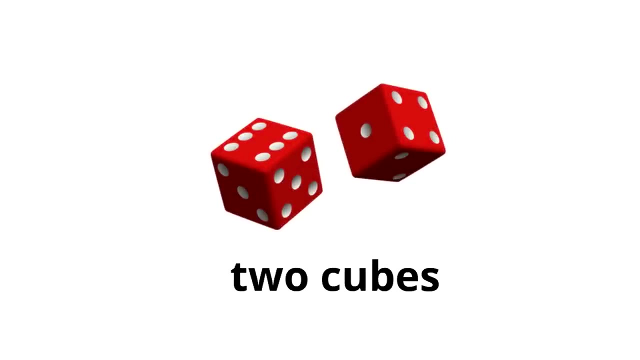 The cube is the 3D version of the square. It has six sides or faces that are all squares. Here we have two dice Dice are in the shape of a cube, So these two dice are two cubes. They have six sides or faces that are all squares. 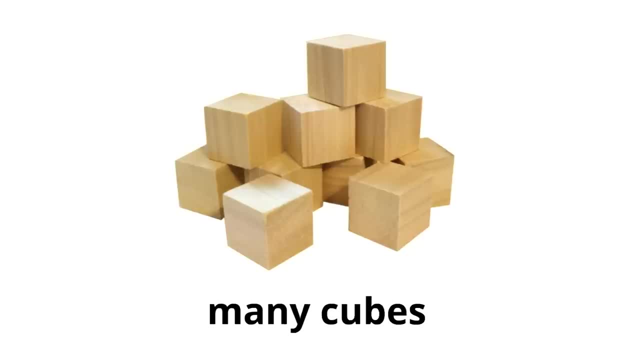 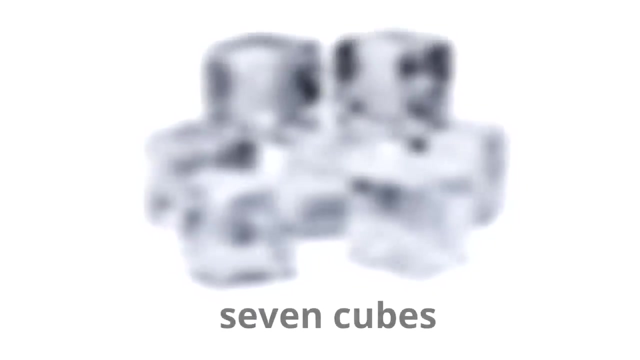 Here we have many cubes. These are cubes that are made out of wood. Each of them have six sides or faces that are all squares. Here are seven cubes of ice. Have you ever had a warm drink and you need to put ice in it? 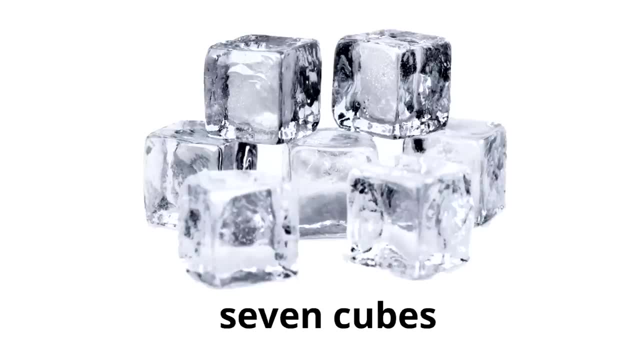 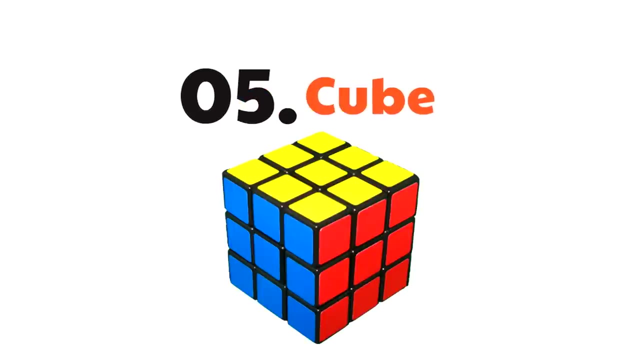 It's awesome because it has this great shape, the shape of a cube, six sides or faces, all squares. I mean, there you go, the cube right, The 3D version of a square, and it's got squares all along the sides right. 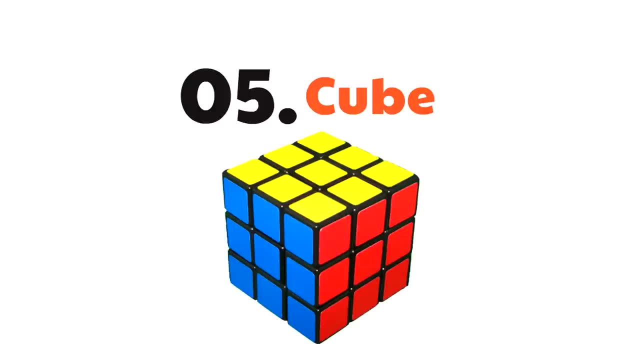 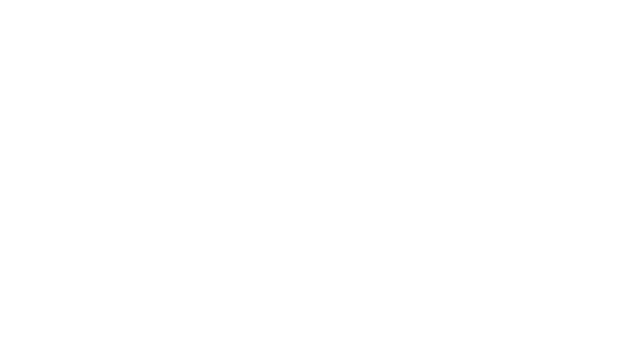 There's six sides or faces all squares, and I don't know. I think it's a pretty cool shape. Our final 3D shape is the rectangular prism. The rectangular prism is the 3D version of the rectangle. It has six sides or faces that are all rectangles. 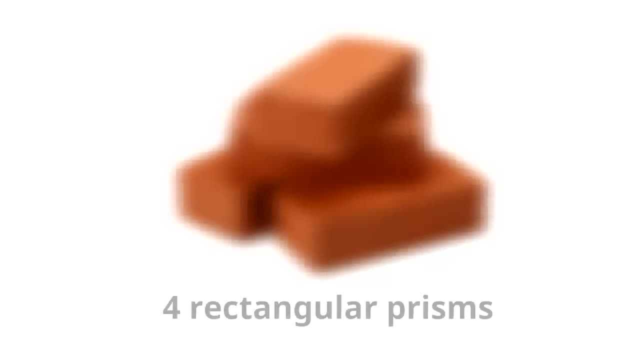 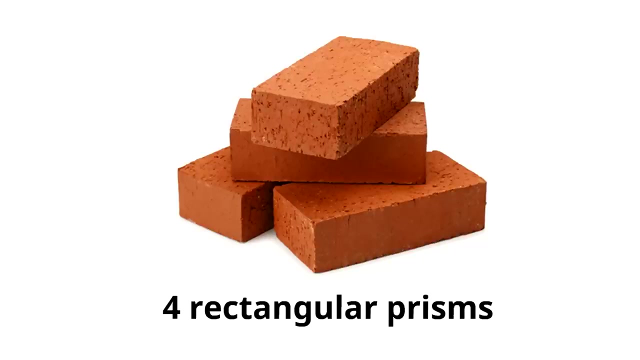 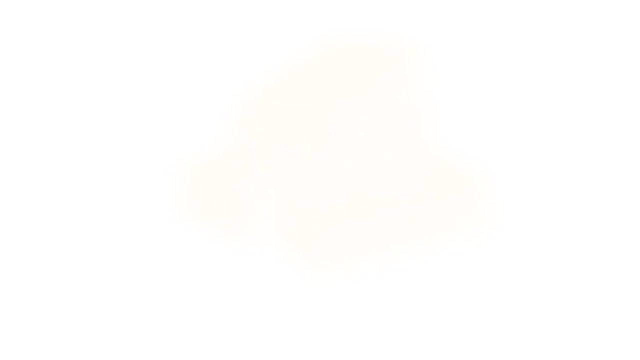 Okay, an awesome example of the rectangular prism are bricks, And here we have four bricks which are four rectangular prisms, The 3D version of the rectangle. Oh, Oh, Oh, I haven't seen this in your classroom or in your home. it's a Kleenex box. 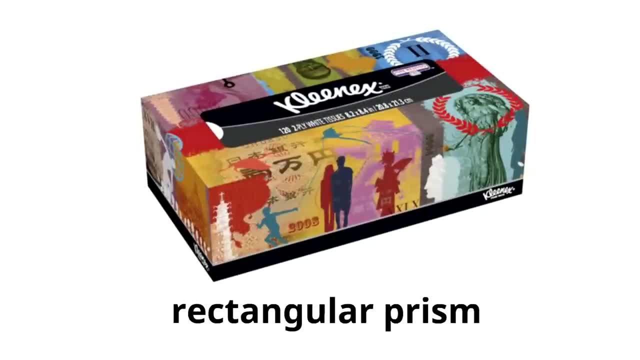 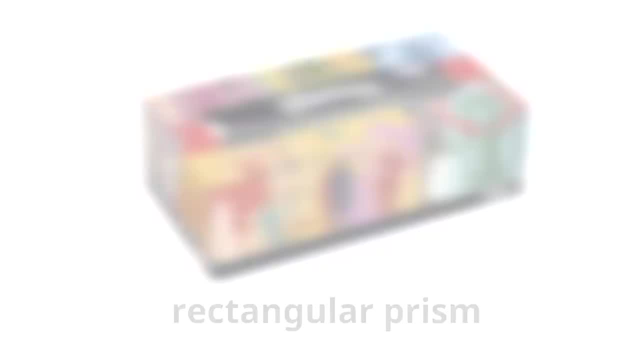 And the Kleenex box is a great example of the rectangular prism. It's got six sides or faces that are all rectangles. Okay. so the secret is, most boxes are rectangular prisms. So here's another rectangular prism, and it's a box. 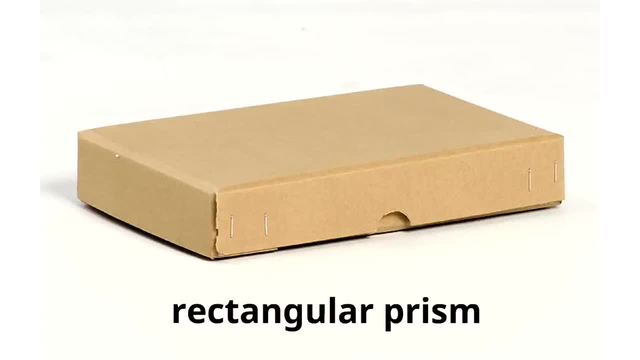 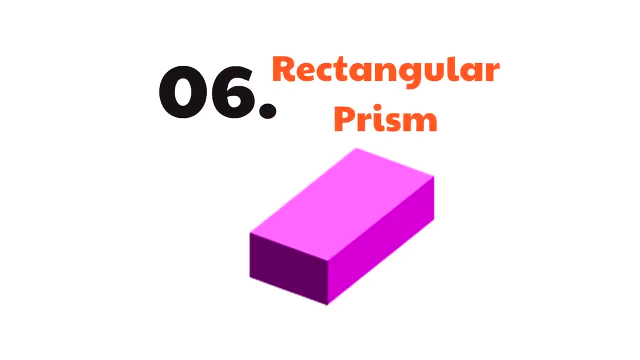 And it's a shorter box, but it still has rectangles all around and it's a rectangular prism. what else can we say? it's a cool shape. the rectangular prism is the 3d version of the rectangle. it has six sides, or faces, that are all rectangles, and it's just a neat. 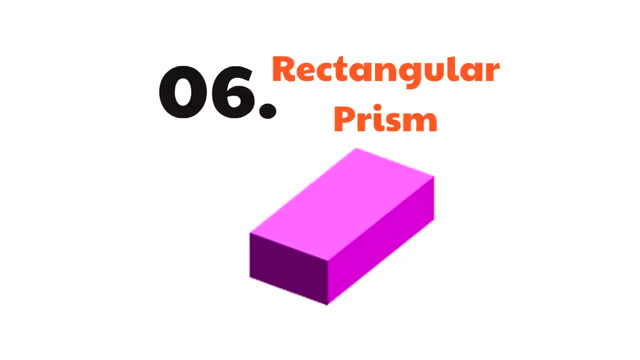 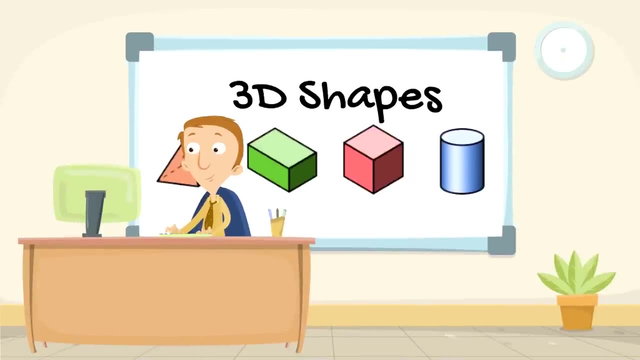 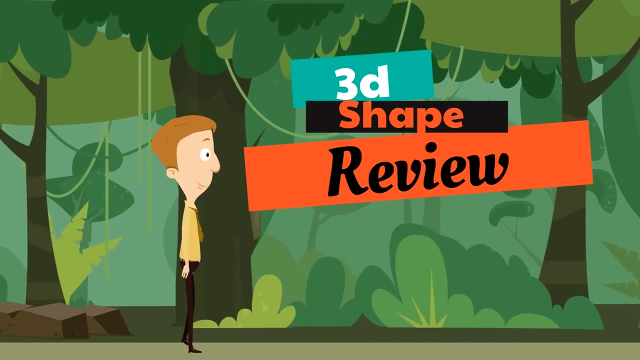 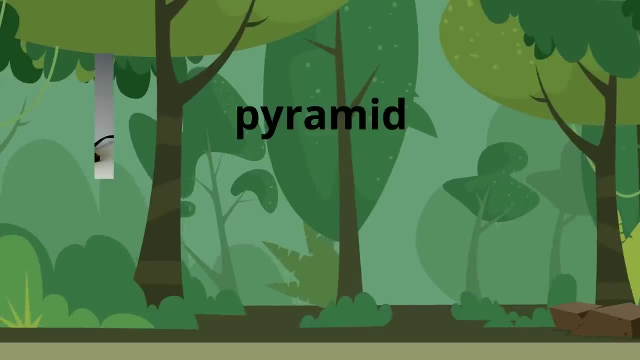 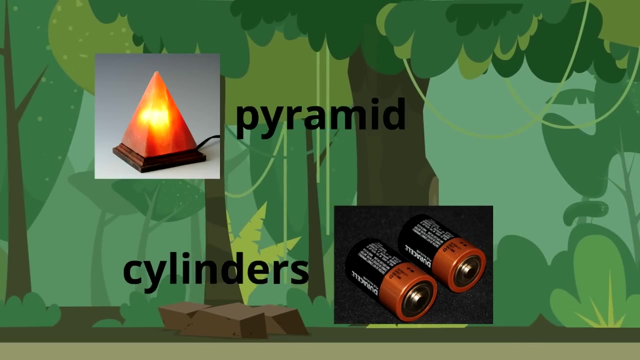 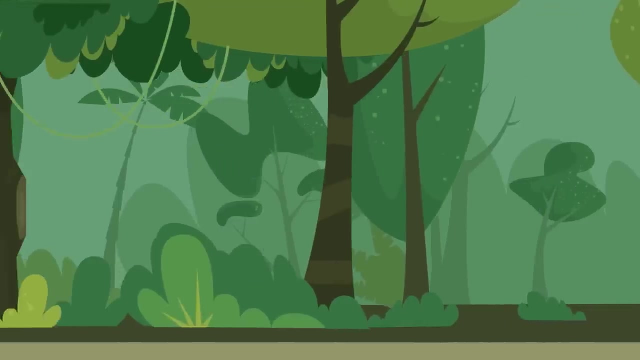 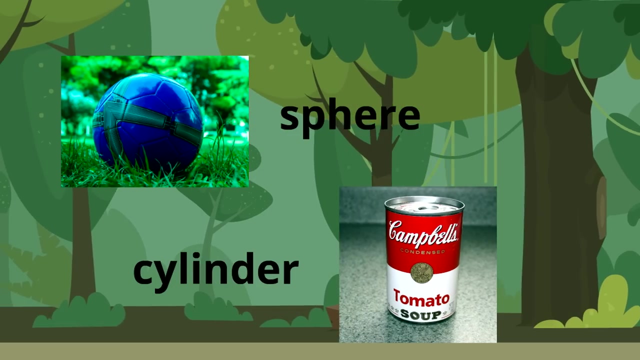 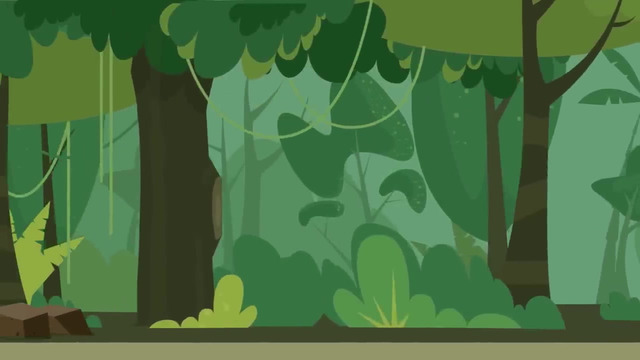 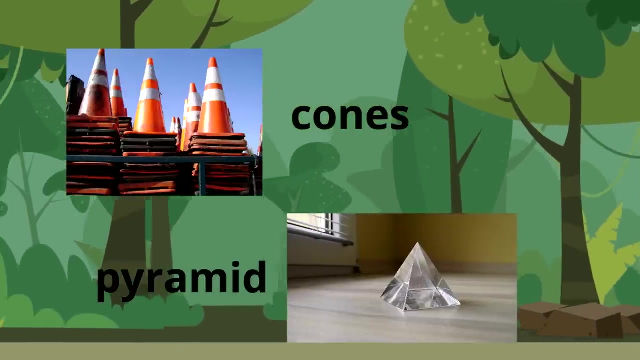 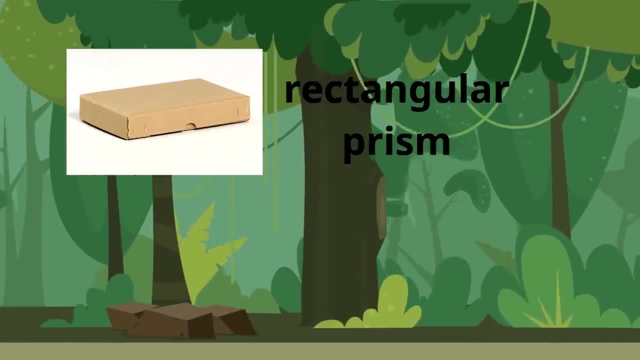 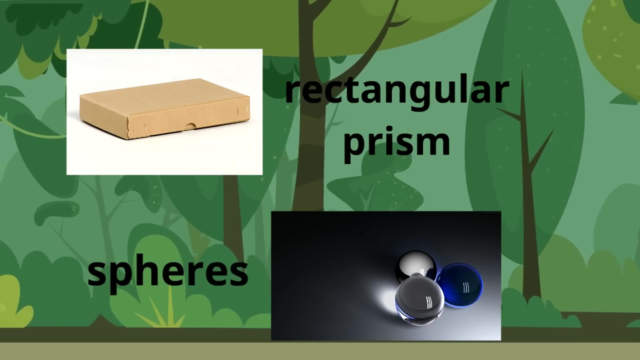 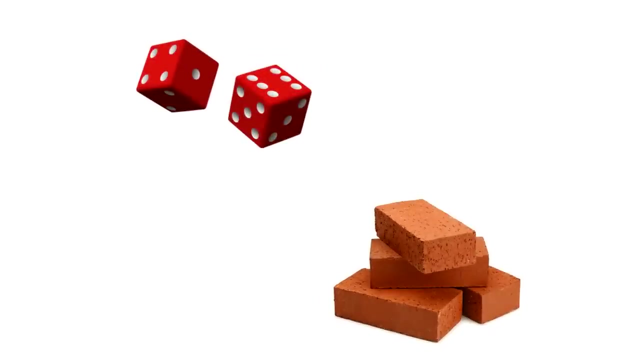 shape to have around. i think i mean you know it's cool, hey? so let's review it. pyramid cylinders, sphere cylinder cones, pyramid rectangular, prism spheres- let's do some more. let's do some more. let's do some more. on the top, here we have cubes. we can tell that because it's the 3d square. it has six sides. 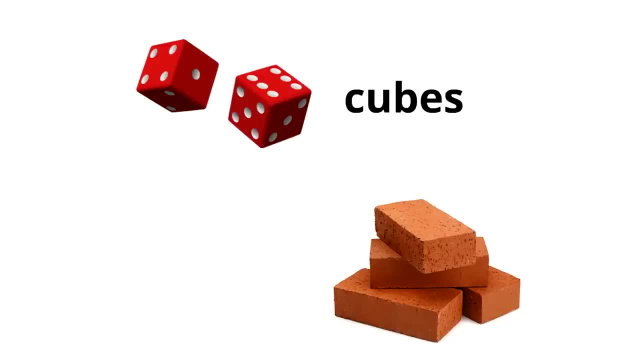 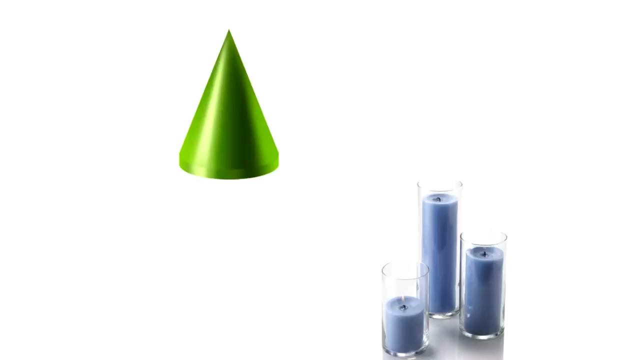 or faces. each of them are squares. it's pretty cool. do you remember what shape these bricks are? yeah, a rectangular prism. they are rectangular prisms. they're the 3d versions of the rectangle. at the top we have a square, we have a cone, a cone, it's got a circle base on the bottom and all comes up to one point called 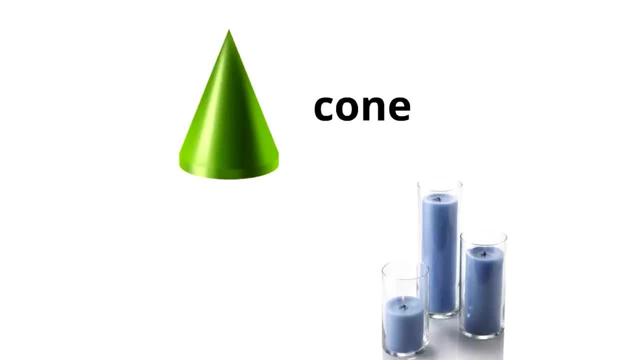 a vertex. do you remember the shape here on the bottom? these are three cylinders. they have a circle on the top and a circle on the bottom and it's smooth all around. you're doing such an awesome job, seriously so cool. so what's this top shape? do you remember? 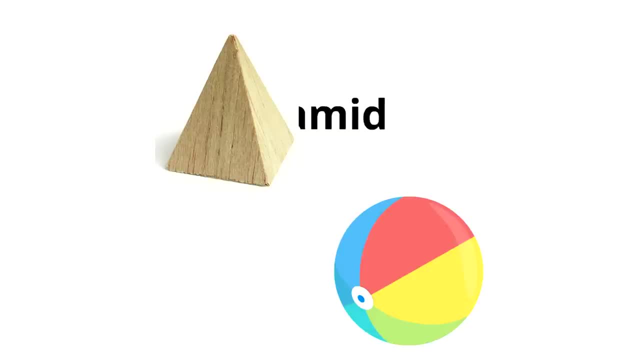 yeah, it's a pyramid, a pyramid. a pyramid has a square base. it comes up to one vertex or one point, and has triangles as the sides. all right, do you remember this last shape here on the bottom? yes, it's the sphere, the sphere which is the 3d circle, and we started with it and we're ending. 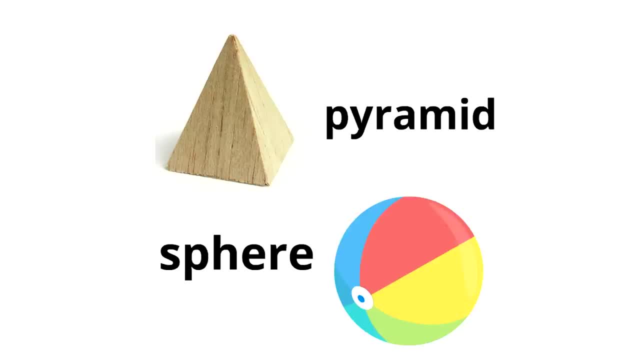 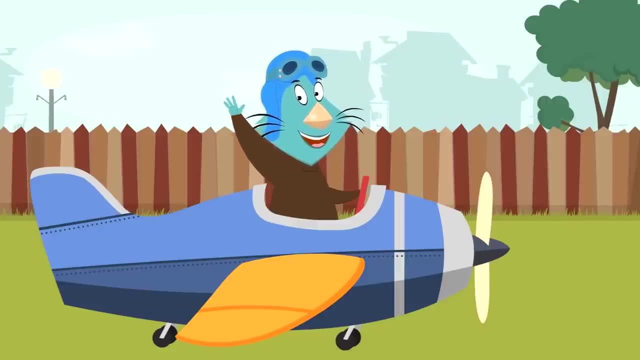 with it and it's so awesome. hey, pd, i know, i know i heard about your plane. you know it's a cool plane, you know, and, and it's, it's neat. i don't know if it flies or you. you look pretty confident that it's gonna fly, which is cool. yeah, i see you, hello, hello. yeah, thanks for waving. 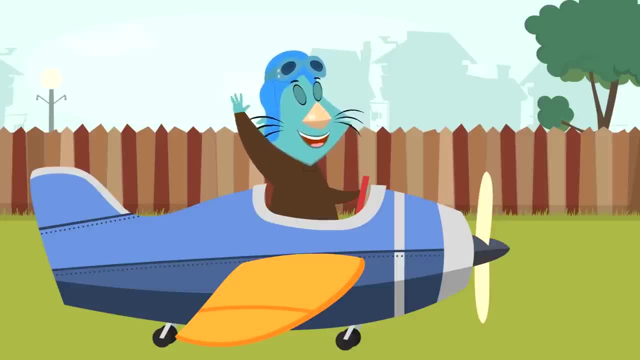 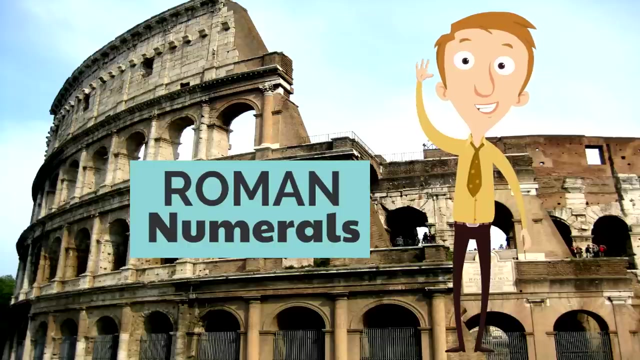 thanks for saying hello. you know, we're actually in the middle of learning. we're we're in the middle of learning a lot of new cool things right now, so i actually do have to go. hi, you're still waving, okay, um, we're gonna go, uh, because now we need to learn about roman numerals, which is a different. 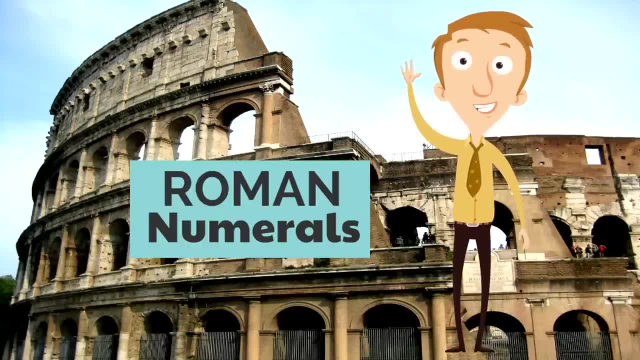 way to write numbers and it was used a long time ago in ancient rome and it's been used since then, and you can think of it almost as a secret code way of writing the numbers. it's pretty simple to learn and we're going to go through that. 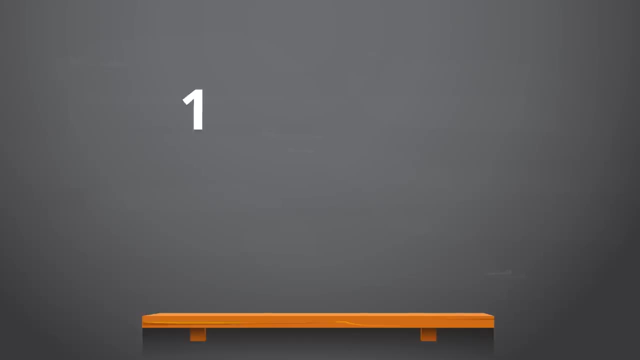 the first roman numeral we're going to learn is the roman numeral i and i is one. i equals one, so if you see an i with a roman numeral, it's one. the letter v is the roman numeral, that means five, and the letter x is the roman numeral. 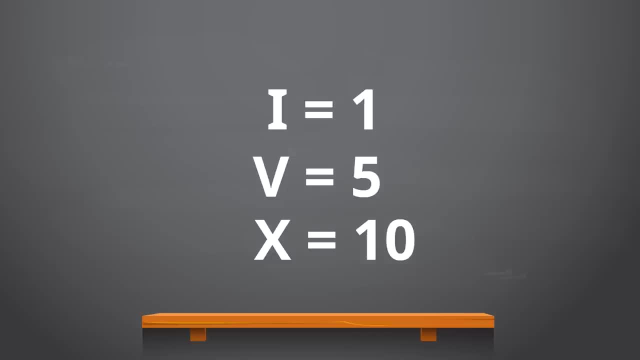 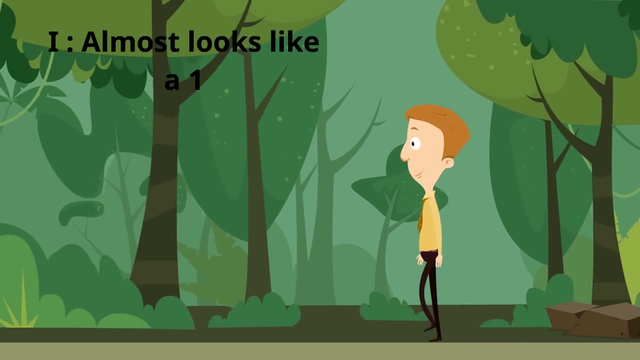 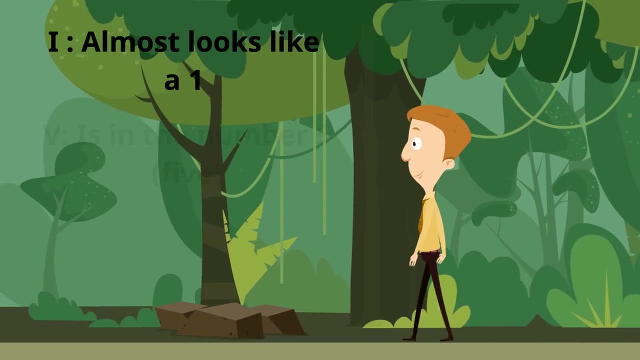 means ten. so when you think one it's an i, you think five it's a v, and if you think ten it's an x. so that's it, just those three i. it almost looks like a one. that's how you can remember that i is a one. i is the roman numeral for one. a v is in the number five. when you spell it out, the 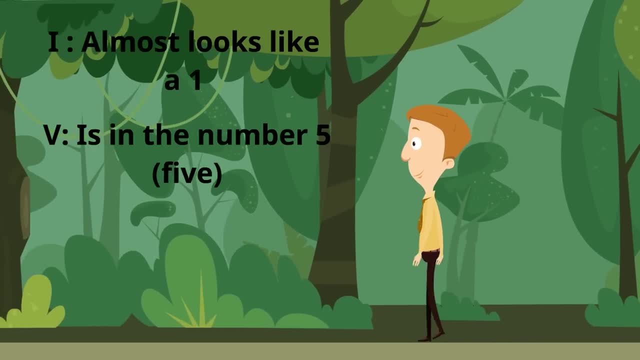 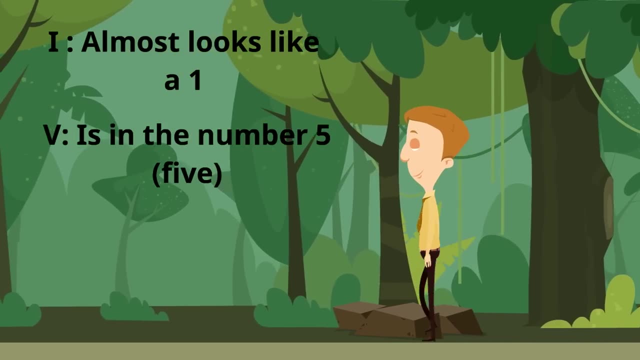 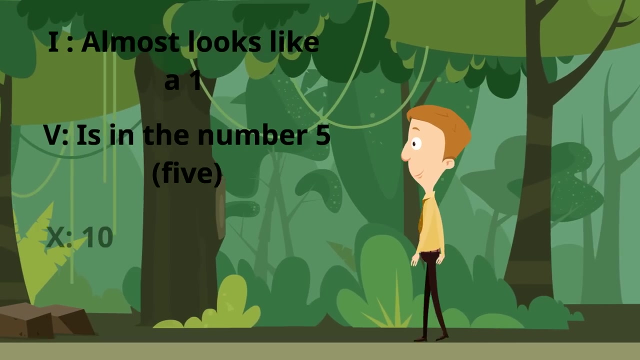 number five. you see that right there, it has a v in it. so when you think of v, you know, oh, you know what. there's a v in the spelled out number five. so v has to be five. now ten is x, and we can't think of anything that could remind us of that. so there is no memorization thing. 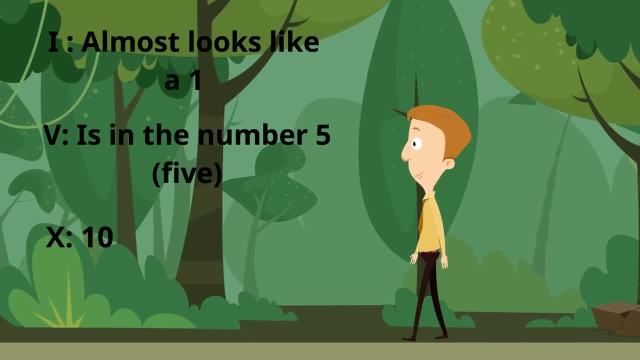 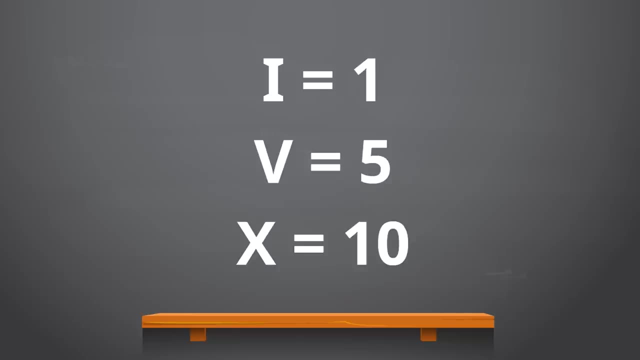 just when you see the x, it's ten, and that's just what we're gonna have to do. okay, one last time here. i just want to make sure you get it. there's only three. i is the roman numeral for one, v is the roman numeral for five and x is the roman numeral for. 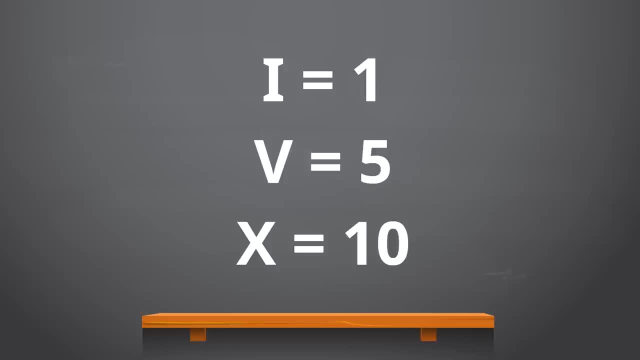 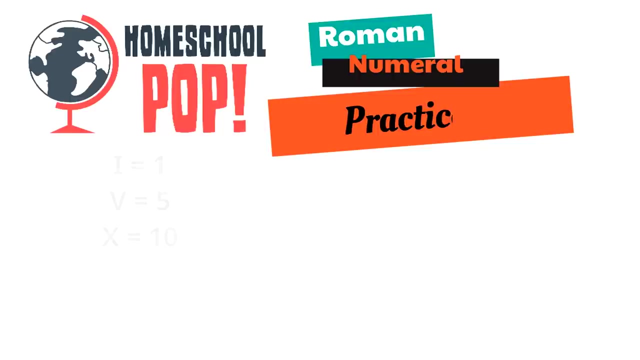 ten, and you gotta understand that so that we could start playing kind of a game of putting them together and making numbers other than just one, five and ten. so let's get started. so let's practice putting these roman numerals. what number do you think this is? you see two eyes and I is one, so the answer is two, two eyes. 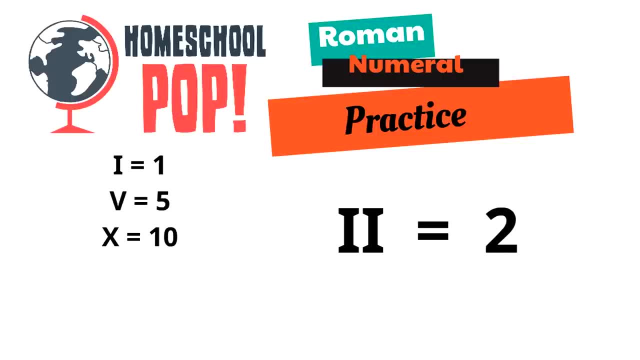 is the number two. what about this one? what number do you think this is? there are three eyes. yeah, it's the number three. let's try this one. what number do you think this is? we see two X's, and X equals 10. so 10 plus 10 equals 20. great job, this is the number 20. 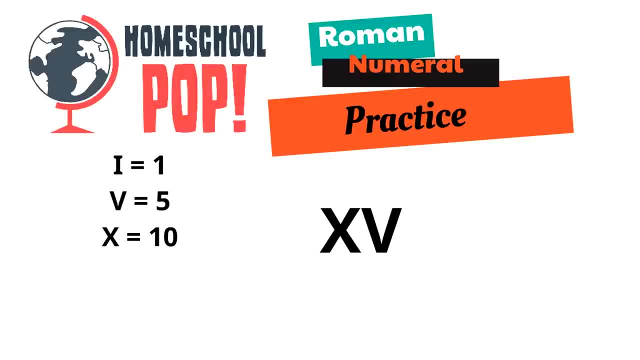 whoa, this one is so cool. okay, an X and a V. what number do you think this is? the X is a 10. the V is what number? five, awesome, so what is? 10 plus 5? 15? whoa, thanks so much for helping out. now that we've looked at how to put some of these together, I want to tell you about two. 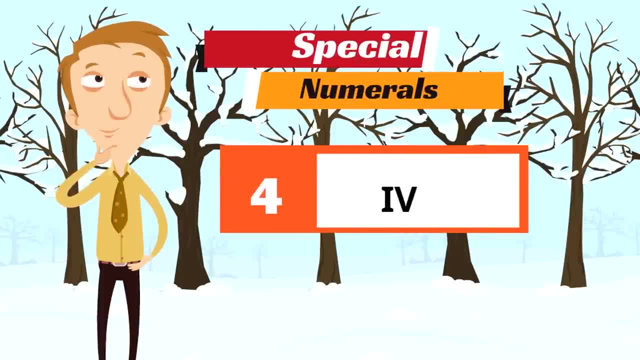 special numerals that are a little bit different, and so you're going to have to just remember these on their own. the first is the number four, and the number four is represented with an I and a V, and the I is before the V, because four is one less than five, which is V. so remember with